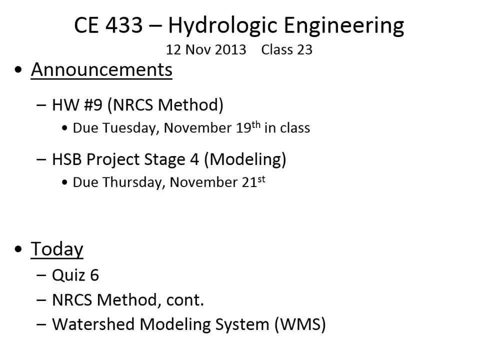 Any questions related to the announcements. I don't know. It really won't be important for you to have in your hands during the final, I don't think. But I'll grade it. I'll grade it as quick as I can. It's tough to say this far in advance what other things I'll have going at the time. 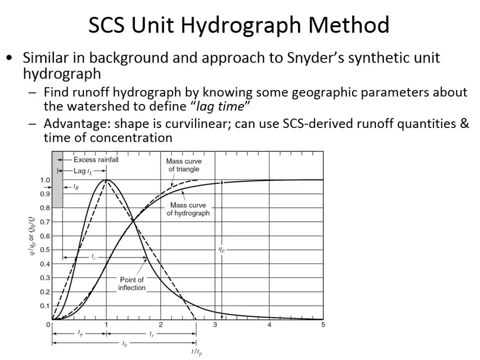 All right, today we're going to talk about one last unit hydrograph method, and this SCS unit hydrograph method is really useful and it's the one that we'll incorporate into our watershed modeling most often, because it defines just a single parameter based on the dimensions of the watershed. 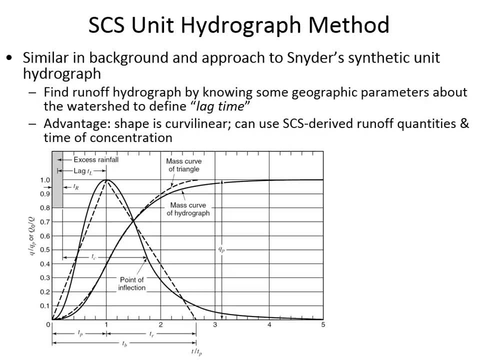 It's the lag time parameter, and then the entire shape of the hydrograph is based off of that lag time that's defined. The advantage of it over other unit hydrograph methods is it's curved, linear, meaning that it actually has inflection points and some curvature to it, rather than strictly being triangular. 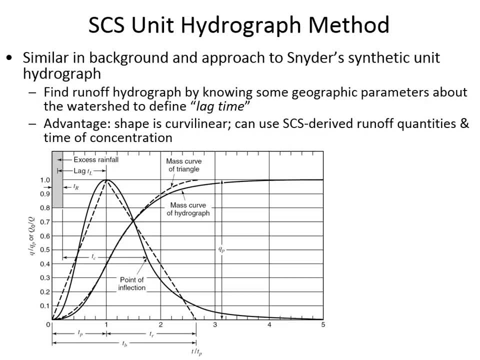 It's based on the triangular shape, but they've put a little bit more thought into it and, having studied a lot of watersheds, They developed this SES method and there are a couple of correction factors depending on if you're applying it in a typical watershed or an urban or a very flat rural. 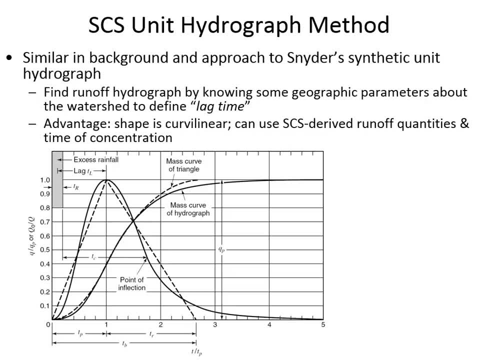 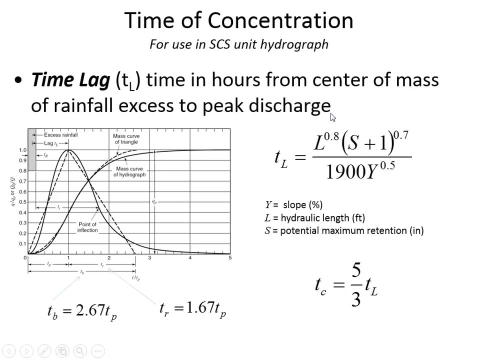 There are a few adjustments that can be made, but ordinarily it yields very good results and all that it takes is calculating the lag time and everything sort of falls into place from there. The lag time is based on a couple of parameters. First of all, you'll notice S, which is the watershed storage. 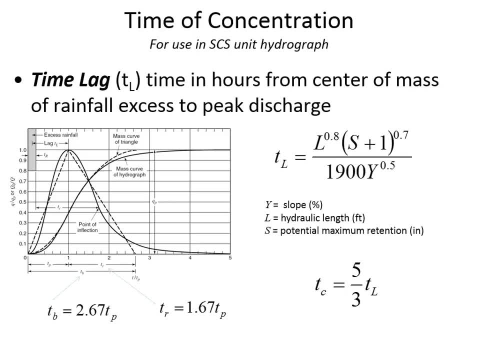 And so the shape of the hydrograph is going to be: basically, how long does it take for the water to go from the start of the storm up to the peak flow? So this T sub P- the time to peak- is a function of the lag time and the time of concentration. 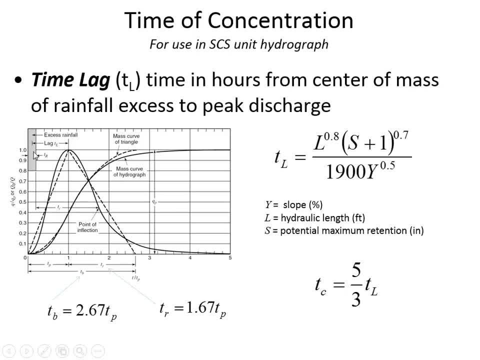 They're all interrelated. They're very slight definitions. You can see that the lag time is from the middle of the rainfall hydrograph, So the duration of the excess rainfall to the peak. That's the definition of lag time. And then there are some the definition of the triangle just sort of builds from there. 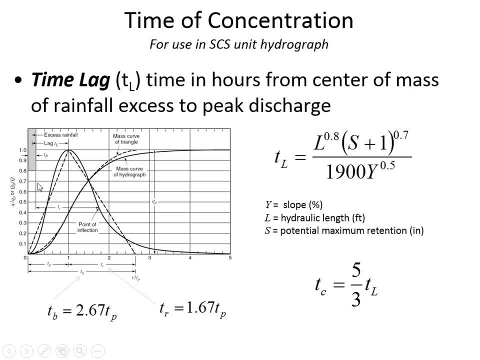 The time of concentration is from the end of the rainfall event to the point of inflection, where the slope is going down and the peak is going down And then it starts, it finishes its decreasing and starts increasing again, that point of inflection. 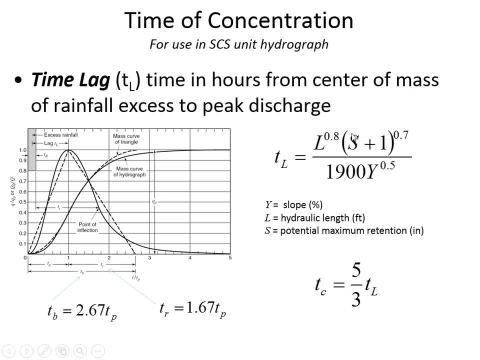 But, as I mentioned before, it's based on the storage And so, of course, from last time, that's a function of the curve number. The watershed slope has a variable here, Y, And so the steeper the watershed slope that's going to reduce the lag time. 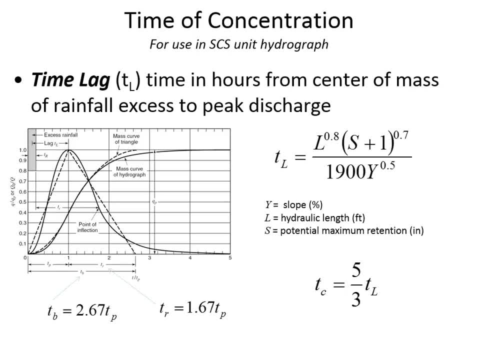 It's going to increase how quickly the watershed makes its way towards the outlet. And finally, L, the hydraulic length is the, the pathway from the furthest point in the watershed to the outlet, And that includes both overland flow, shallow concentrated flow and channelized flow. 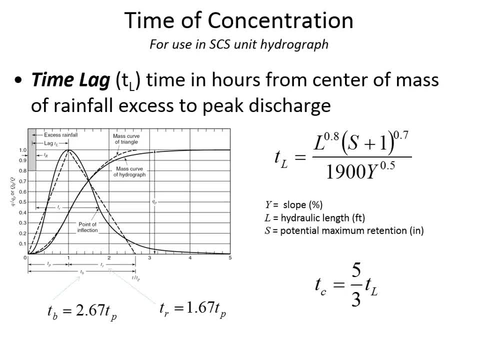 And we can calculate that a lot more accurately using computer tools In the past. they just have to estimate the hydraulic length, because it wouldn't be possible to trace every single path in the watershed to know what's the furthest point from the outlet. It may not be the furthest point in the watershed. 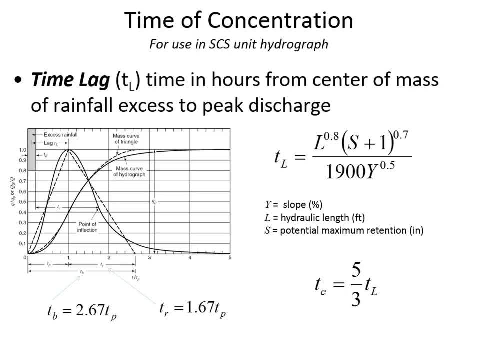 It may be the furthest point as the crow flies, of course There's going to be some meandering paths of the water going towards the outlet. So when we do introduce WMS later today, all of these are parameters that are just reported automatically. 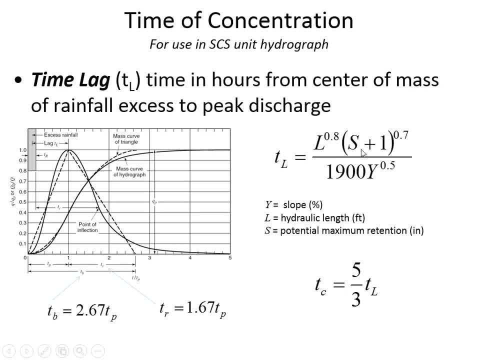 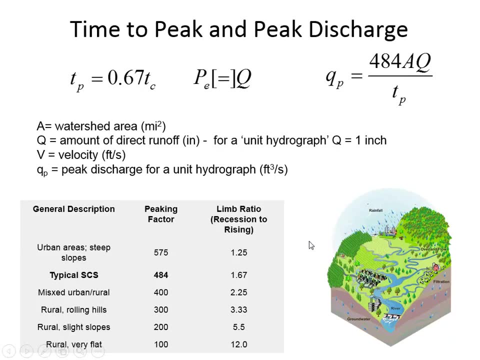 The watershed slope it gets from the underlying elevation data, the curve number It can get from the soil type and the land use data that we read in from GIS data sources. And the hydraulic length is largely based on the GIS data. So once we know the time to peak, we can calculate the magnitude of the peak. 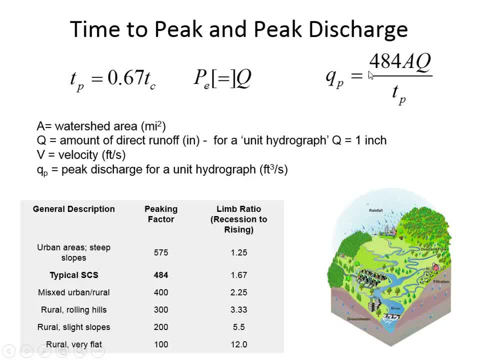 And here's the formula that allows us to calculate the magnitude of the peak. This 484 unit conversion factor here is related to just a typical case when we're applying the SES method, the typical peaking factor. But if you are in an urban area or a rural area, 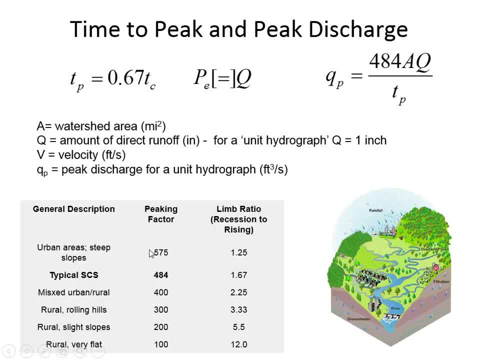 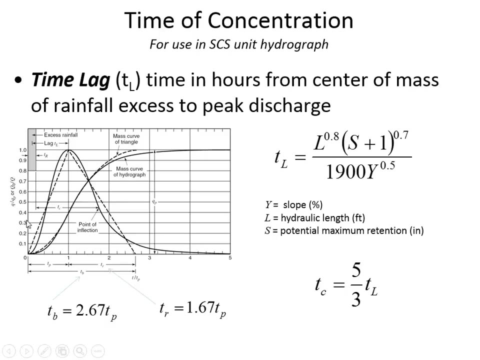 or anything in between. there are a variety of peaking factors that can either increase or decrease the magnitude of the peak runoff. Ordinarily, what we're going to be doing is we're going to be using the shape of this and we're going to be using SES to calculate the times. 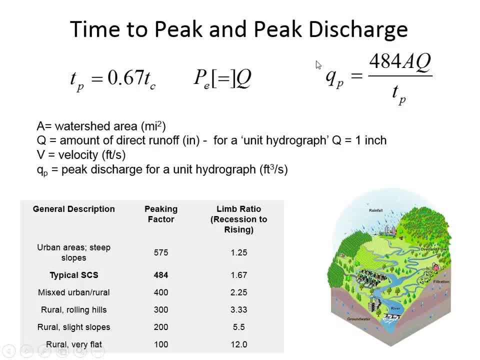 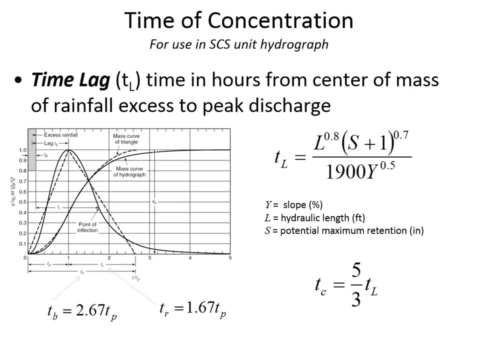 But the actual magnitude of the peak. we won't often use this aspect of the SES method when we're doing watershed modeling in the computer. So in other words, what we're going to incorporate of the SES method into our computerized watershed models is just how long it takes from when the rainfall event starts until we see the peak flow. 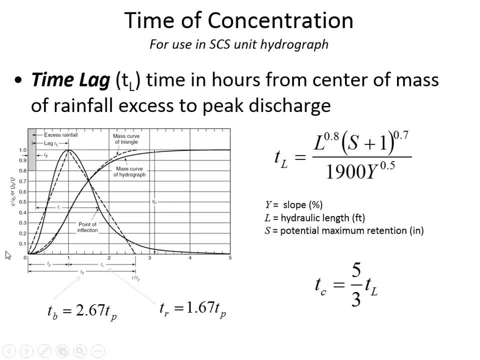 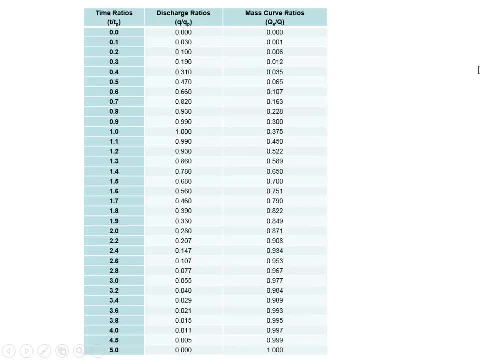 So we'll use the SES method to identify the relative shape of the hydrograph. And let me jump ahead just quickly to show you these mass curve ratios and the discharge ratios, Once you have the time defined, the SES method, the time to peak defined. 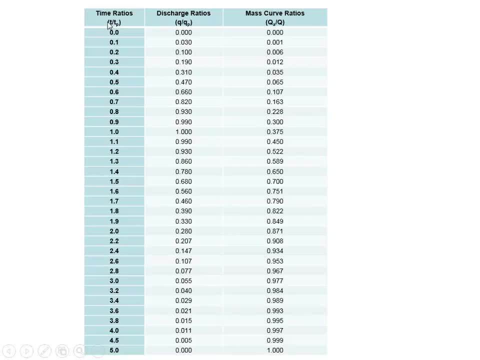 so 1.0 is the time versus the time to peak, And so if it takes three hours for you to see the peak flow, then that's at 1.0. And 2.0 would be six hours. It would be two times since you started the storm. 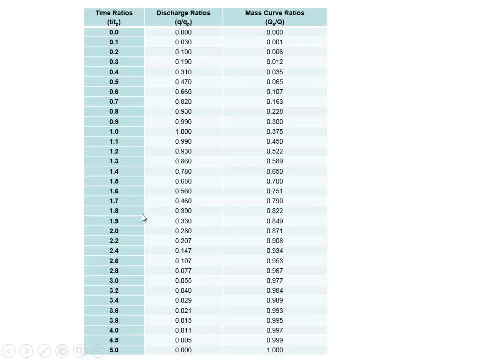 In other words, another time to peak after the first three hour storm. So the discharge ratio is just telling you. of course, 1.0 is the peak itself, but at 1.1 times of the time to peak it's 99% of the peak flow, and so on. 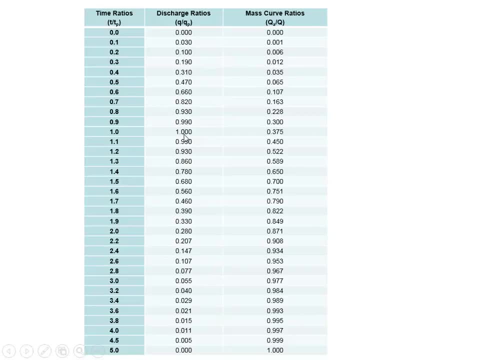 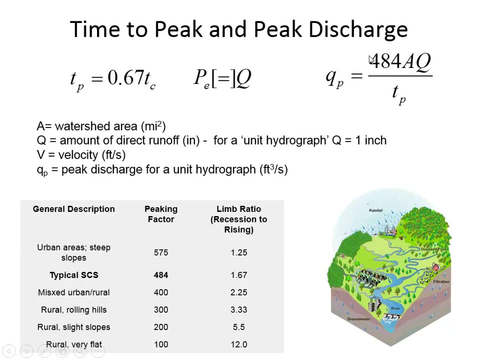 So this tells you how long it takes to get back down to a zero flow, And so we're going to be using the relative shape of the unit hydrograph, but not necessarily using the SES method, to calculate the magnitude. We'll do that here in an example, here, in just a minute. 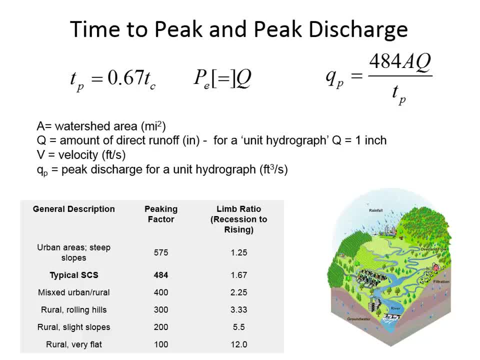 We'll use this SES method all the way to its conclusion to find the magnitude of the peak, But we have a more sophisticated approach to find the magnitude, and so, then, we only rely on it for the relative shape, In addition to adjusting the peak of the hydrograph. 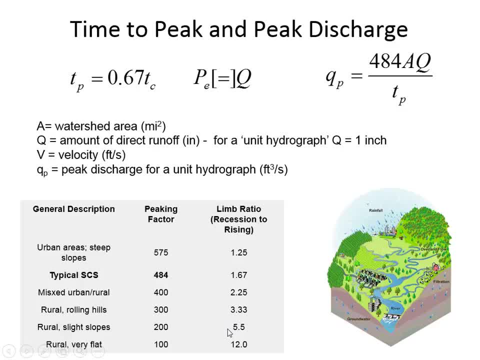 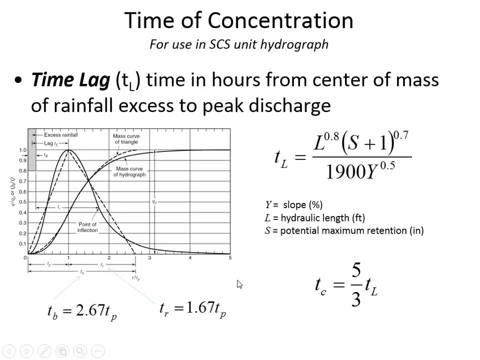 we can use these adjustment factors to say how much longer it's going to take to drain the watershed. So the 1.67,. if you'll notice, in the previous slide we said that the T sub R, so they call that the receding limb. 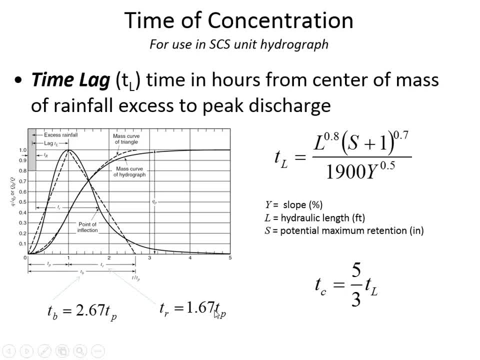 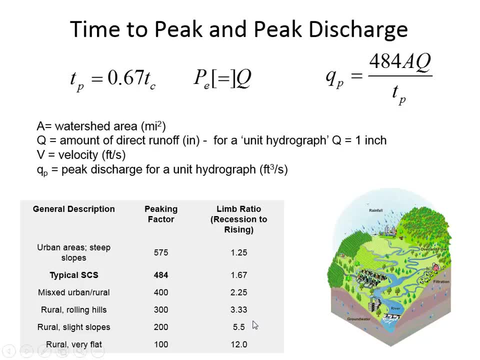 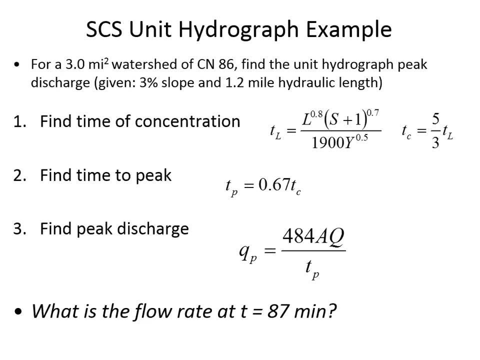 is 1.67 under ordinary circumstances, but if you have a watershed that's going to drain very slowly, then you can use these multipliers to extend how long you're likely to see flow coming out of the watershed. All right, so let's put this into practice for a three square mile watershed. 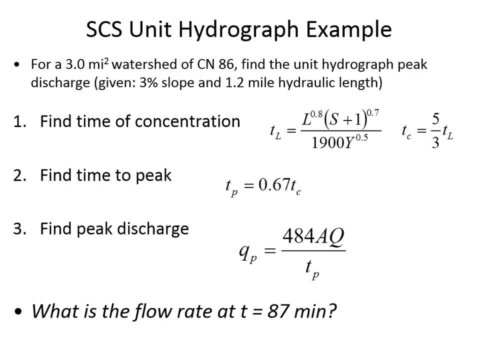 We know the curve number and the slope and the hydraulic length, and so those are going to be able to allow us to define the time of concentration. One thing to keep in mind is that the slope should be in percent, so Y should be equal to three. 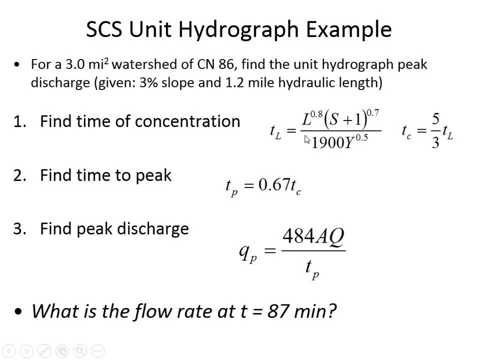 but the hydraulic length needs to be defined in terms of feet, And so put the length of 1.2 miles, convert that into feet to find the T sub L and the T sub C. And then the other thing is that the A 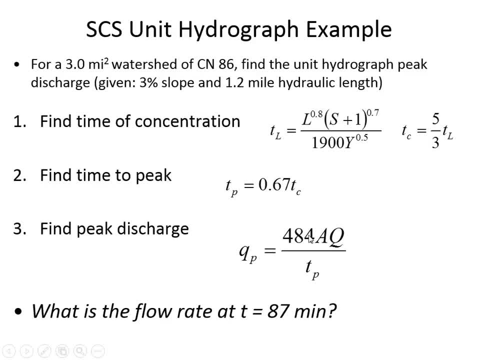 the units of area are in square miles, and so go ahead and do steps one through three and then together we'll find out what's the magnitude of the flow rate at 87 minutes And assuming one inch of rainfall, because it's asked for find the unit hydrograph peak discharge. 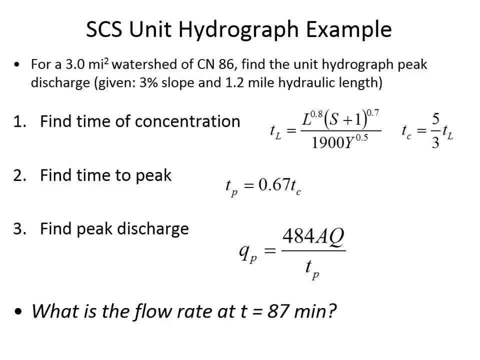 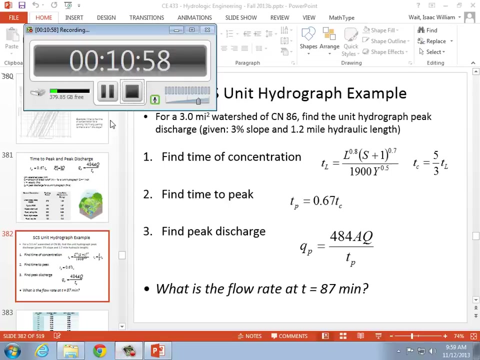 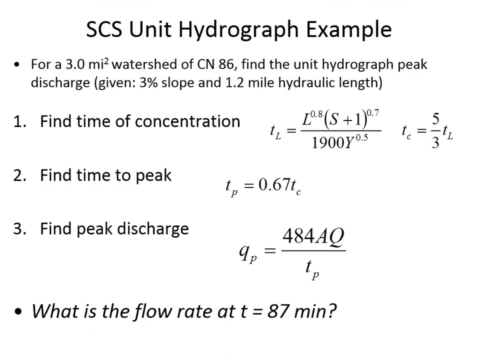 so, assuming one inch of rainfall, one inch of rainfall excess, that is Okay. we find the time of concentration by first finding the lag time, which is 0.656 hours. The S we can find from the NRCS formula, 1,000 divided by the curve number minus 10,. 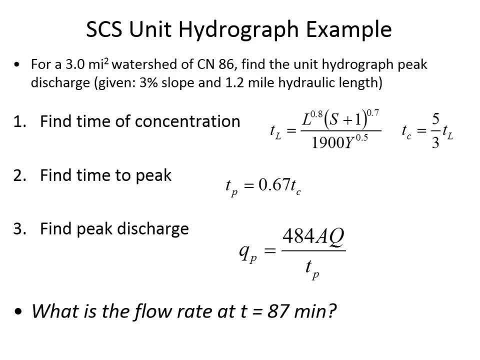 that gives us 1.63 for the S. Converting the hydraulic length from miles into feet, it's 63.36 feet and three as the percent that we substitute into Y, So that 5 thirds times the lag time is 1.093 hours for the time of concentration. 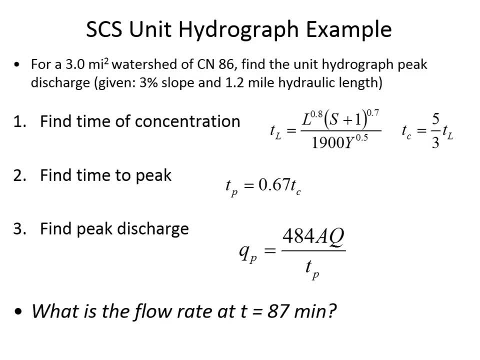 Once we know the time of concentration, we can calculate the time to peak, and the time to peak is 0.729 hours In this case. just for illustration purposes, we are using the SDS approach to find the peak discharge, and that turns out to be 1992 CFS per inch. 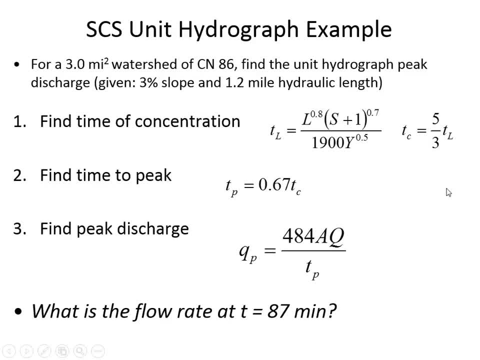 and the reason why Q was given as one inch is because we said by definition that this is a unit hydrograph and so we assumed one inch of rainfall excess. So for every one inch of rainfall excess that happens, we're going to see 1992 CFS per inch. 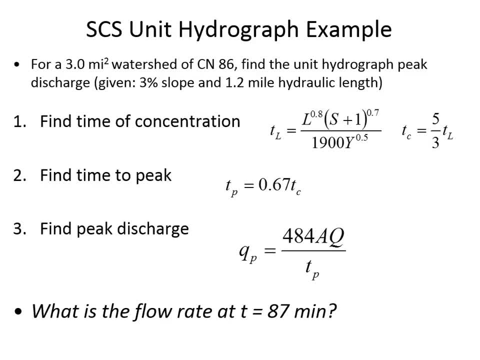 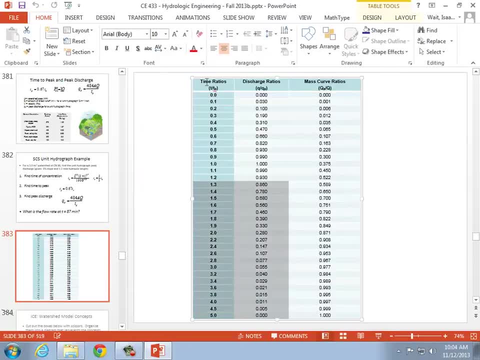 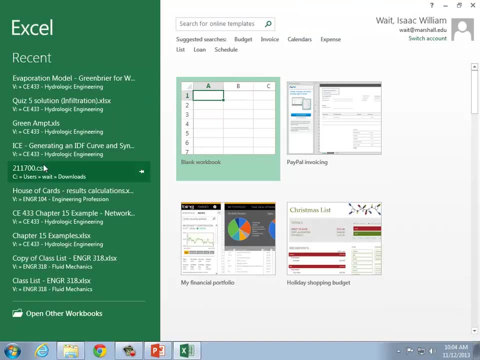 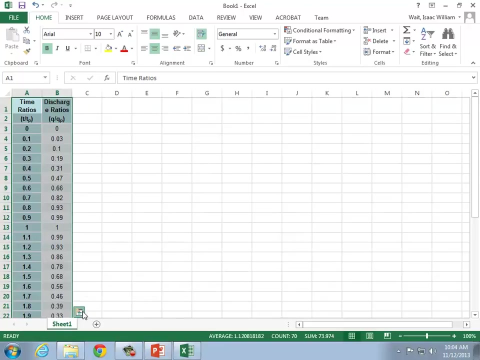 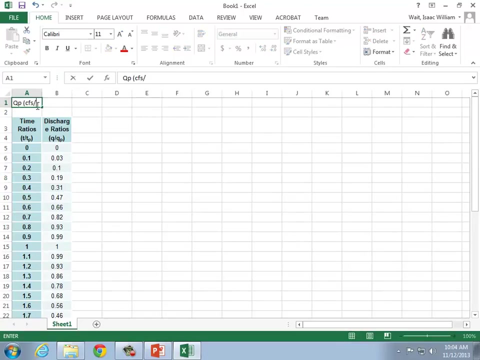 and so when does the flow actually occur? We can take the discharge ratios and paste that into Excel. and we said that the peak discharge is going to be the 1992 CFS per inch, 1992 CFS per inch, and so that the Q at any time. 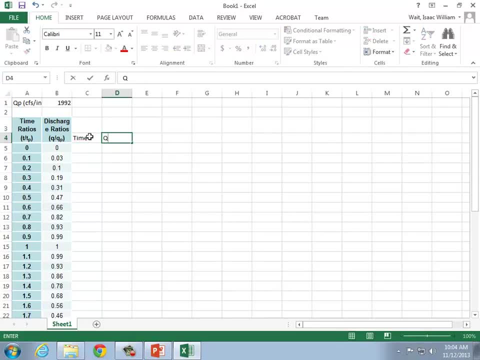 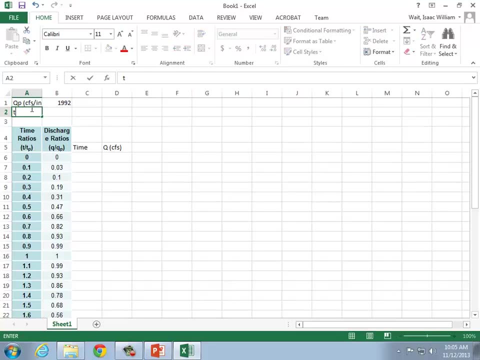 well, actually, maybe we should say what the time is and then have the Q. The time to peak we calculated was 0.729 hours, and so that now these times become absolute instead of just relative by multiplying the time to peak by the time ratio. 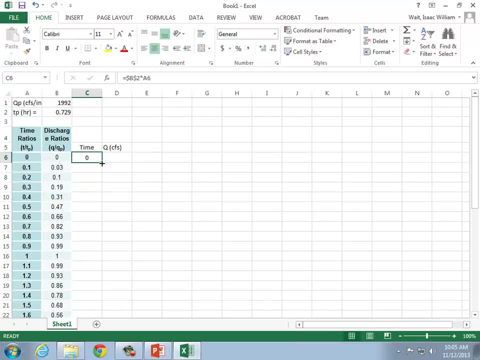 So it's the shape of the hydrograph that we're making use of, and once we apply that shape to the time that we calculated based on geometric parameters, remember that this T sub P is just based on our understanding of the retention inside of the watershed. 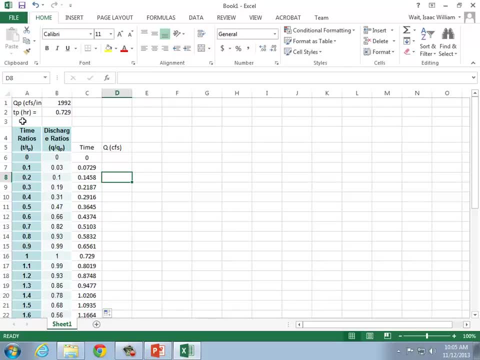 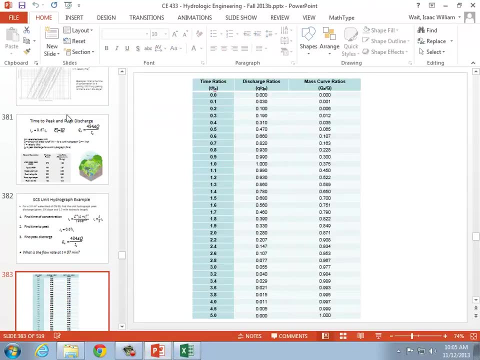 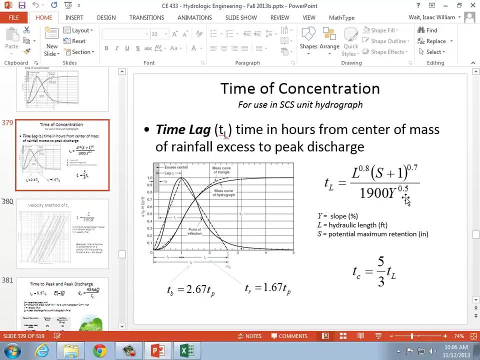 its slope and the hydraulic length, and so a larger watershed is going to have a larger time of concentration because of the hydraulic length being larger, and similarly a very steep watershed will have a smaller time of concentration because the Y parameter in the denominator is going to reduce the value of the lag time. 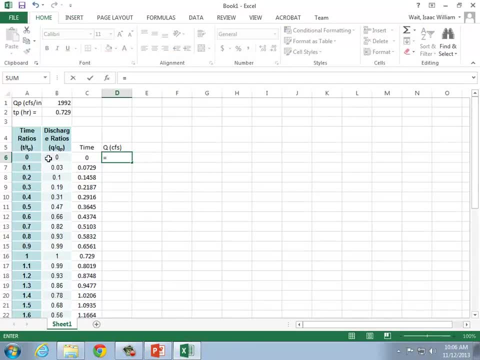 Okay. so going back to this spreadsheet, we can multiply the discharge ratio by the peak and then carry that through and you'll see that we have the peak here at that means that we've got the peak time and the magnitude of the peak. 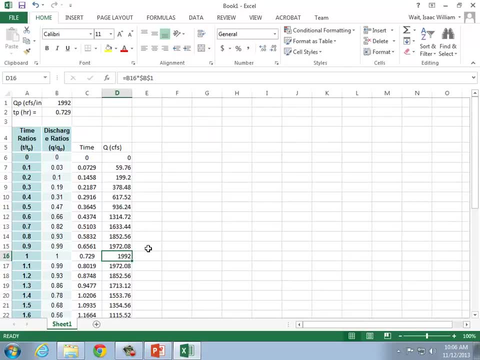 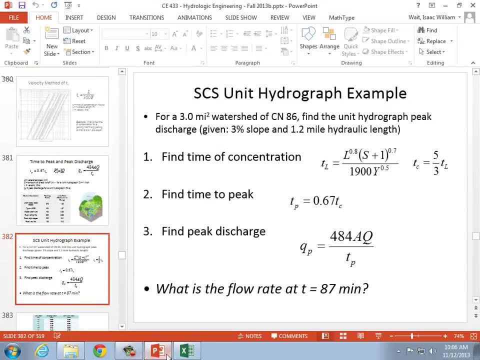 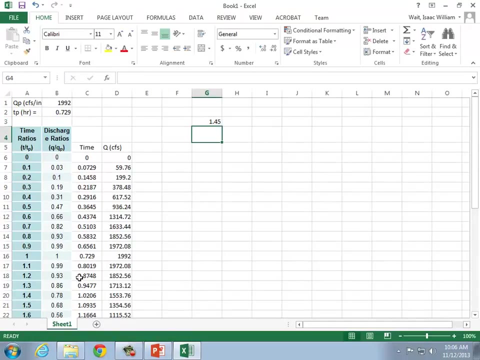 and so we can find out at any particular time what the flow rate is. and in this question it asks at a time of 87 minutes, and so 87 minutes is 1.45, so that would be halfway between these two, and so we could just say it's going to be. 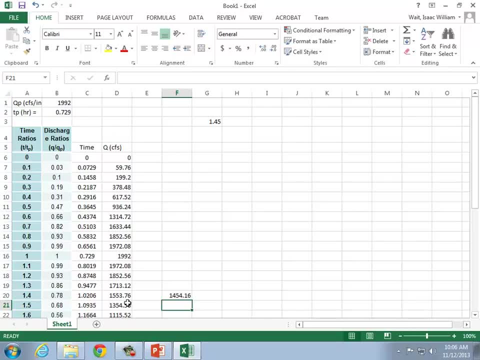 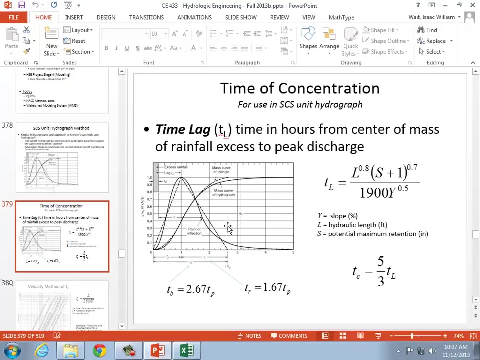 1454 would be approximately the flow rate that we'll expect to see at the time of 1.45 hours. Any questions on that example? Okay, so what we're going to use on a continuing basis is the shape of this curve. 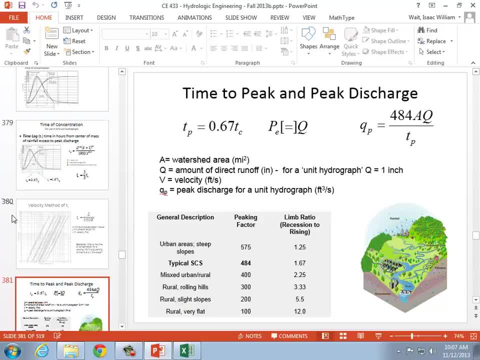 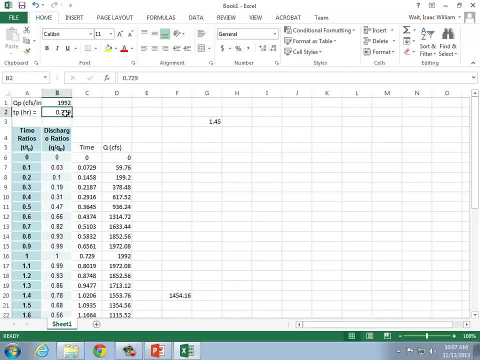 We won't really make use of this formula, and the way that we're going to continue to make use of it is we'll have some other way to tell us what the peak flow rate is. We'll still continue to use the SES method. 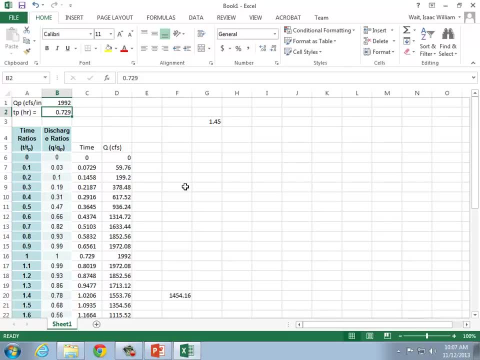 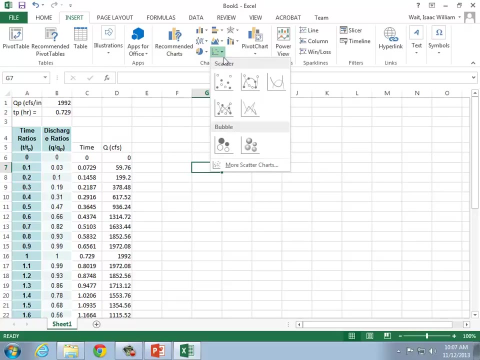 to find out what the time to peak is, just not the magnitude of the peak, and so that doesn't render this any less useful than it already is, because we can scale this and it- let's just draw a hydrograph briefly, it'll just change the magnitude of the hydrograph. 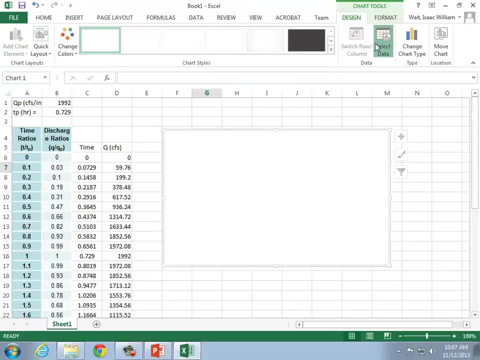 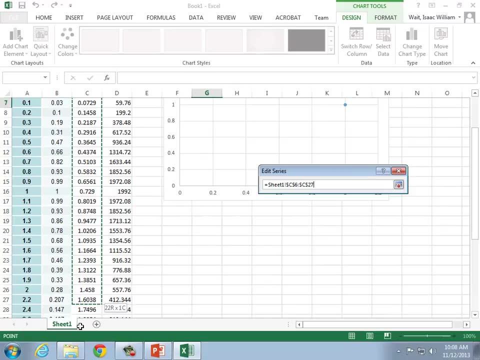 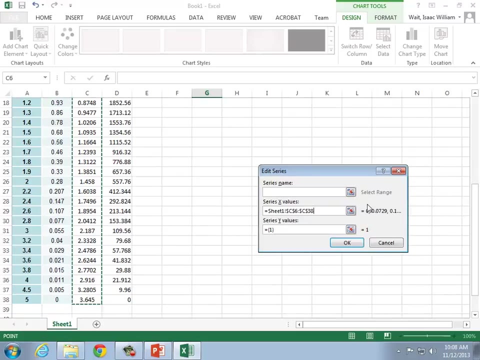 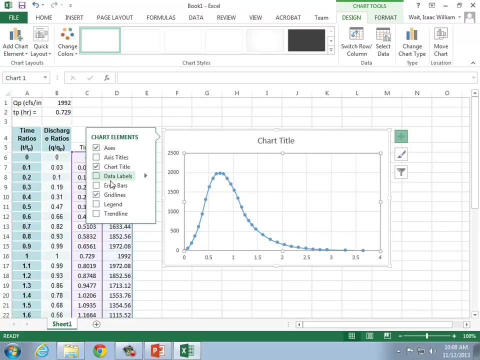 but not necessarily any of its durations. So if we have this being our time in hours, oh, computer's locked up, there we go and the magnitude of our flows, this new way of doing things here. data labels: no, no no. axis titles: yes. 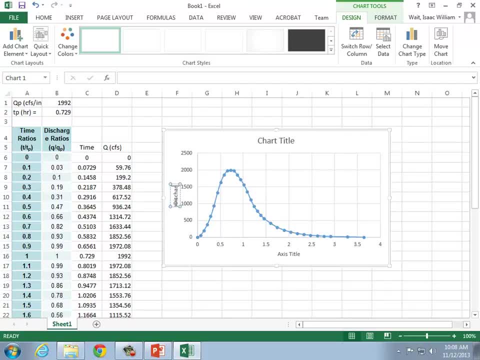 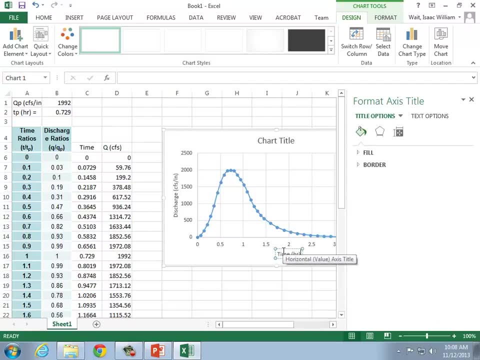 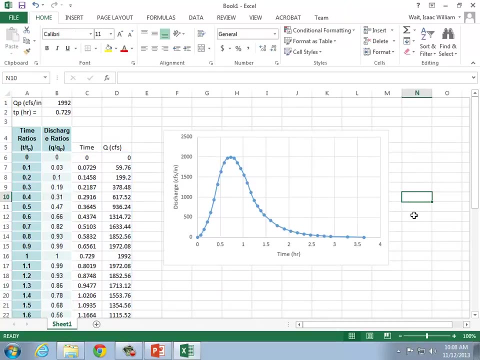 Okay, so this is our discharge and this is our time. When we do modeling in the computer, there's going to be other ways for us to find out what the peak is, more sophisticated than that equation we have, and so maybe the model that we'll do- 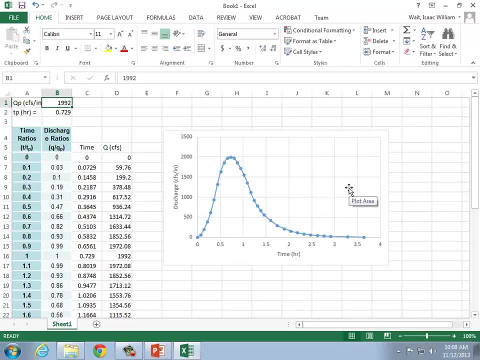 we'll find out that the peak discharge is actually 2500.. So it simply scales the peak, but the relative magnitude at any particular time stays the same. We'll be using that curve linear shape that's defined by the SES method. So any questions about this unit hydrograph. 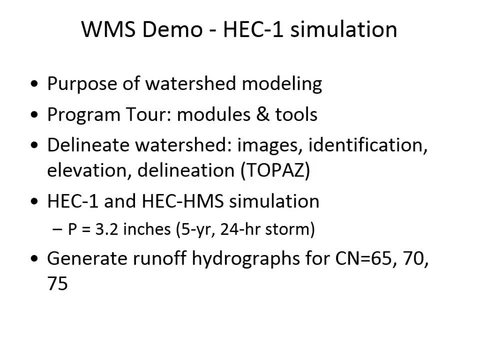 All right, so here it is. It's the meat of the next couple of lectures. It's going to be WMS- the Watershed Modeling System, And if you'd like, you can grab a tablet to follow along. I'm not actually going to ask you to necessarily do anything. 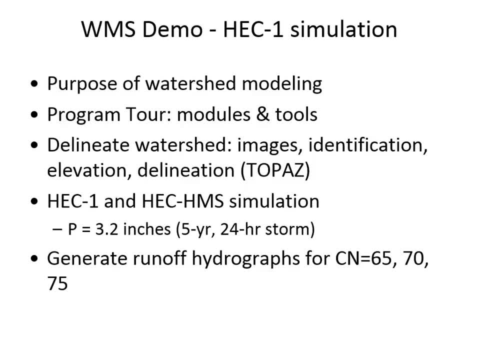 You can follow the demonstration that I'm going to be walking through if you choose, but you'll definitely have time to work hands-on in class on Thursday. So if you want to have WMS on your own PC, install it by Thursday, Otherwise you'll be using one of the tablets. 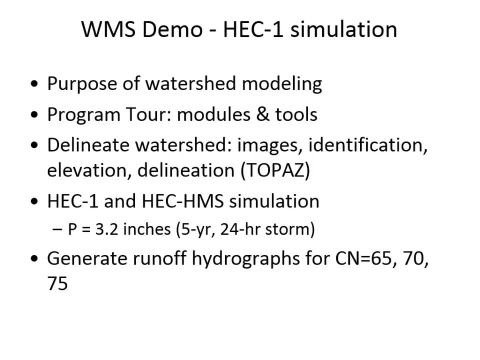 What's that? All right. so I gave you the website address for where you can go on the AquaVeo website to download WMS in the last class and we'll actually go through and activate with licensing and everything, So you won't be able to run the program. 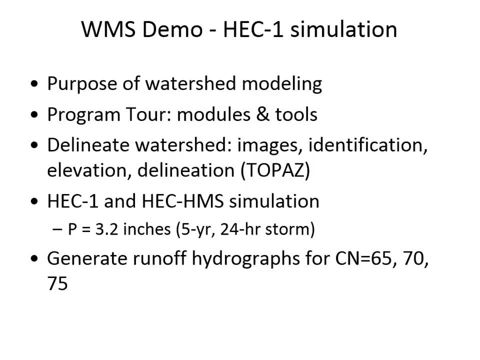 until you have the license code and I'll tell you what that is when we do our demonstration on Thursday together. For now I just wanted to show you a tour of the program and, I guess, talk about the purpose of watershed modeling, why we do it on the computer. 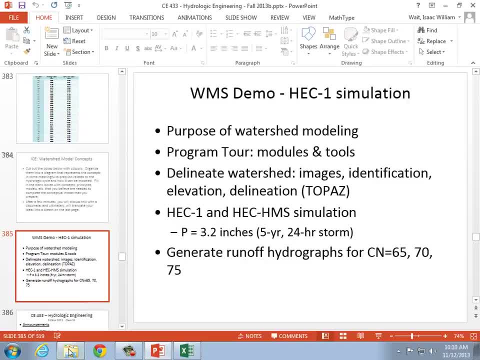 and what sorts of questions it can answer along the way. So I just installed WMS on this and I think it's activated, ready to go. The WMS that's installed on the tablets is 9.0 rather than the new version of 9.1. that's here. 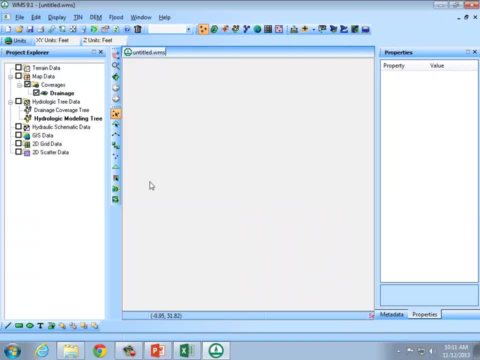 but the differences are relatively minor so I don't think it'll be a problem for us. It has different modules and you can see the buttons along the top here will change depending on what module you are in, and these are the different modules across the top. 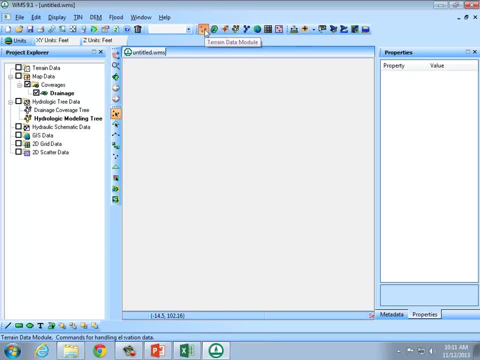 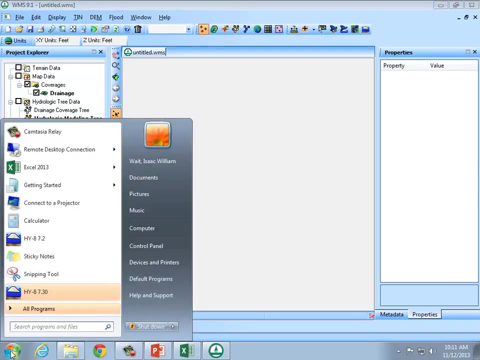 Right now we're in the top right corner. right now we're in something called the Terrain Data Module, and that's a way of interacting with elevation data, because having a map of elevation data in the background is going to be one of the important things that WMS relies on. 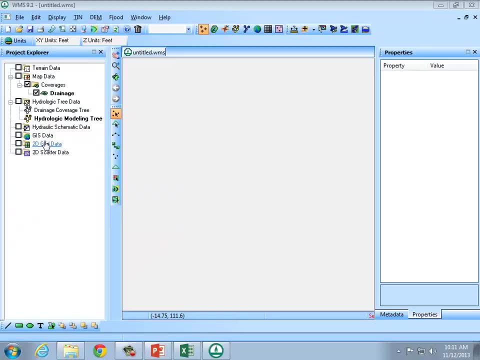 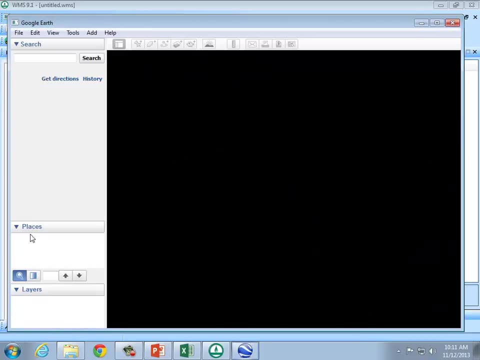 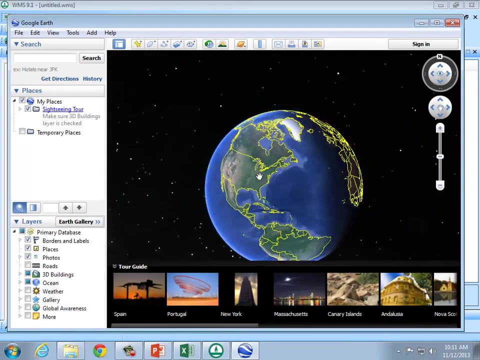 And, whether you know it or not, you've already worked with the DEM. If I open up Google Earth Pro, you've used- I think most of you have used- the elevation data that's in the background on Google Earth To look at the project area that you're doing for your project. 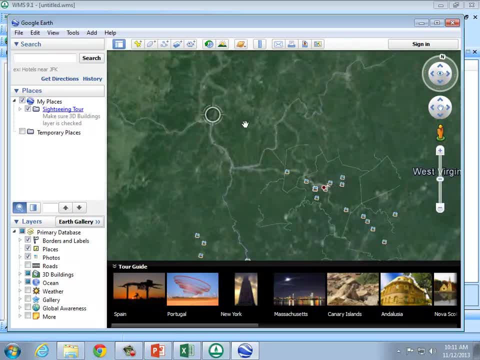 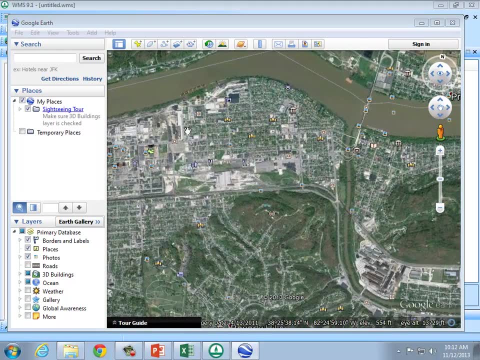 for example. So if we zoom in on Huntington, Alright. so when you just trace the surface, you know down here at the bottom where it says elevation, it is getting that elevation from a digital elevation map. And so when you trace your cursor, 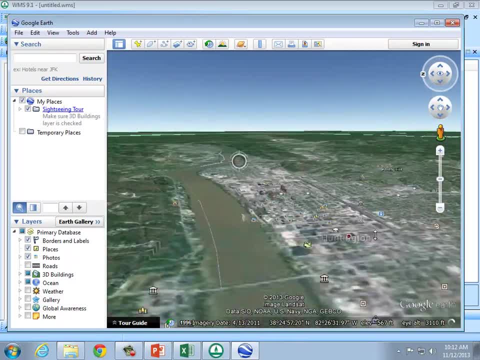 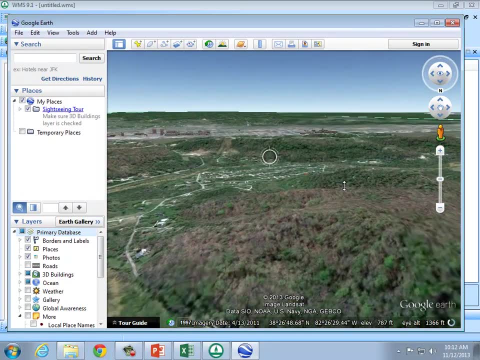 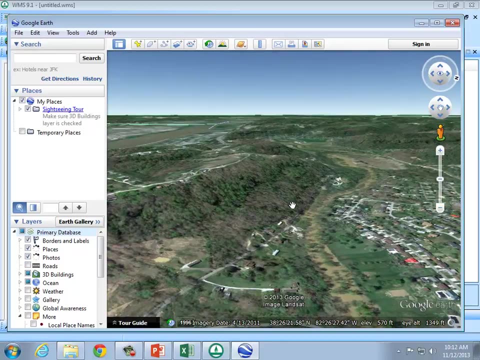 and also when you turn on terrain. Okay, terrain is on. The way that it's able to grab the map and make it appear to have three dimensions is because it has a surface that it's essentially X, Y, Z data at certain intervals. 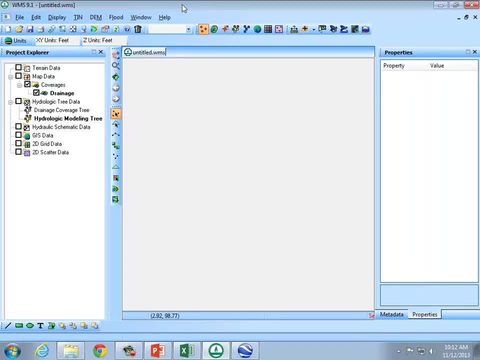 And WMS is going to rely on that X, Y, Z data to not only show that, not only show images in three dimensions, but, more importantly, to delineate watersheds, And so this first module is a way for you to interact. 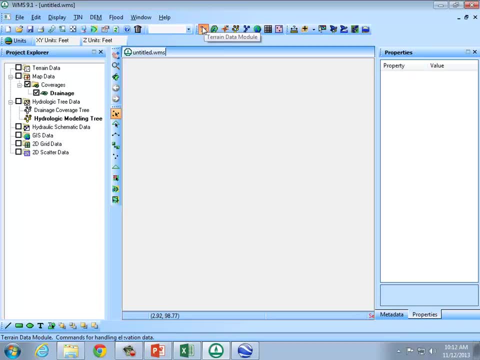 and if you need to manually override some of the elevation data to do that. The drainage module is a way of identifying rivers and streams and sort of setting up where the flow is going. The map module is a is a module that I don't use very much. 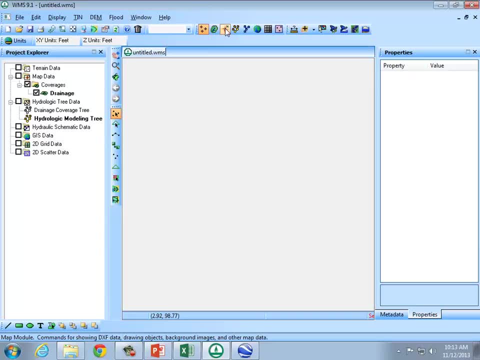 but if you have data that comes from AutoCAD or MicroStation, it can sometimes be successfully imported, sometimes not, but usually for an urban watershed. the map module allows you to interact with the data that comes in from MicroStation and AutoCAD. 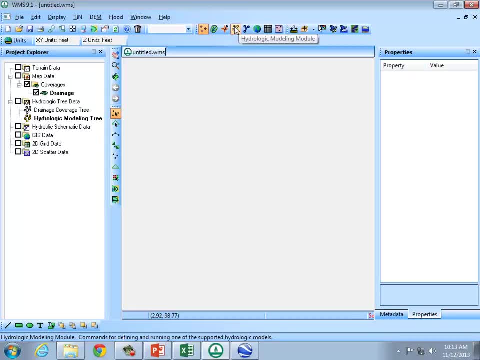 And the hydrologic modeling module is a conceptual kind of module. The tools that come up for that have to do with symbols that you break watersheds up into sub-basins, and so Those are the four main modules we use. These other modules may not even be activated. 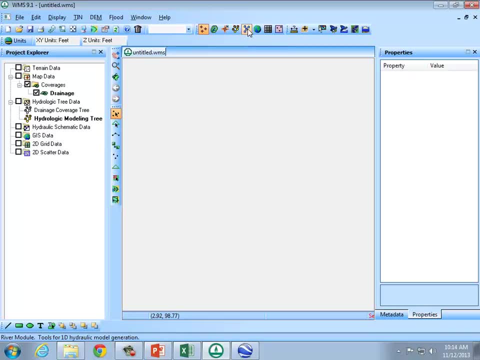 for the license code that I typed in The river module is something you'd use to do heckgrass modeling. It's essentially, you remember, gradually varying flow from hydraulics. It's something that can help you set up a gradually varying flow modeling. 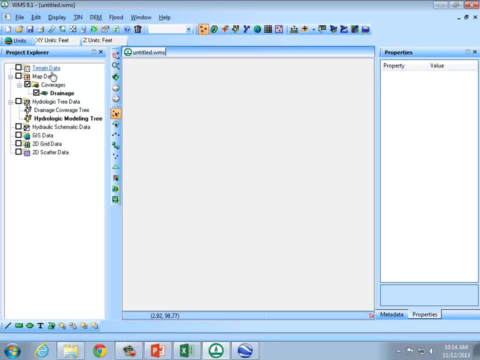 make it a little bit easier when you're trying to do that. So there is a wizard that allows you to step through, piece by piece, the workflow that's required to set up a watershed module, And it's called the hydrologic modeling wizard and it's supposed to look like a wizard's hat. 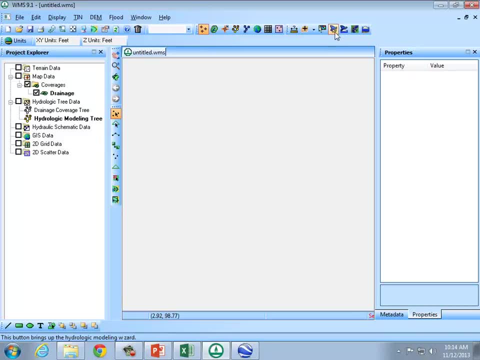 That's what I think the symbol is supposed to be. Now, the little things underneath here might be roller skates. I'm not sure, but it's like a wizard hat on roller skates, So they're making it seem like it's really easy. 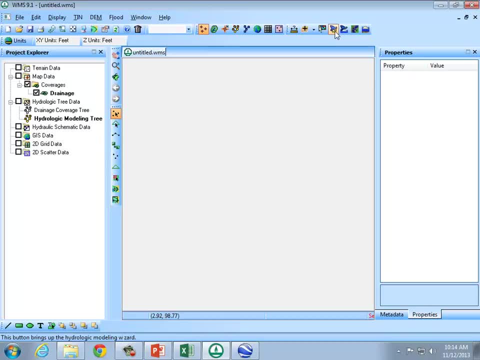 And it is pretty easy if you just step through the things that it tells you to do Over here in the project explorer. this is a way of keeping track of all the different files that you're opening And you know, in StormCAD or WaterCAD. 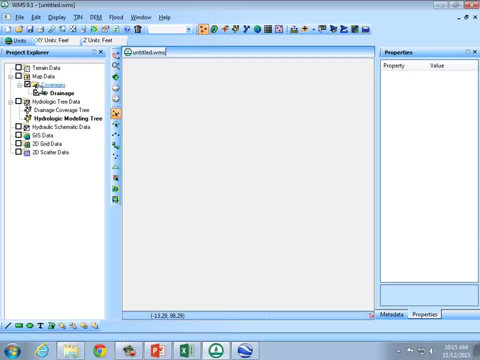 when you save a file, when you save a project, it creates actually four different files and you can't just email one of them and get the project to open. You know there's multiple files that all have different pieces of the project, and the same thing is true in WMS. 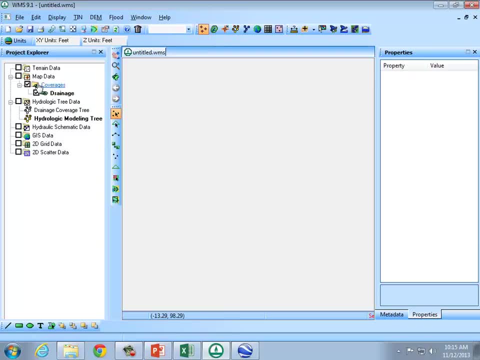 They try to get it all under one wrapper, but you're often going to be opening up external GIS files and this sort of helps you to keep straight all of the files that are going to be a part of the model that you work with The properties window over here on the right. 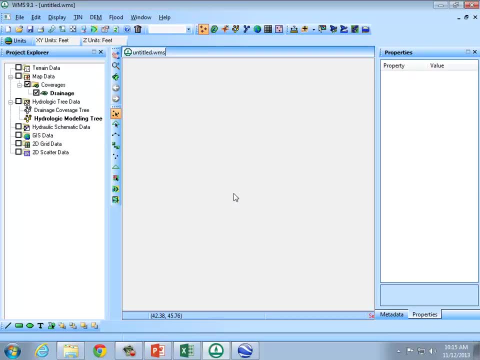 anytime you select an object, whether it is a watershed or a stream, it'll give you properties like how long the stream is, what's the average slope of the watershed, what's the curve number of a sub-basin, and so on, And so this is just sort of where you get metadata. 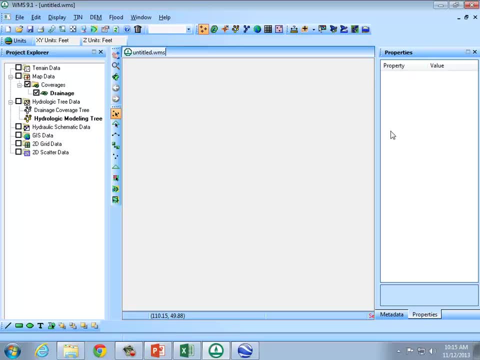 about the elements of a watershed. And then these tools will also vary depending on what module you're in, but these are sort of shortcuts to tools that are also available through the software, So you can go through the menus, you know, to move around. zoom in pan. previous view. 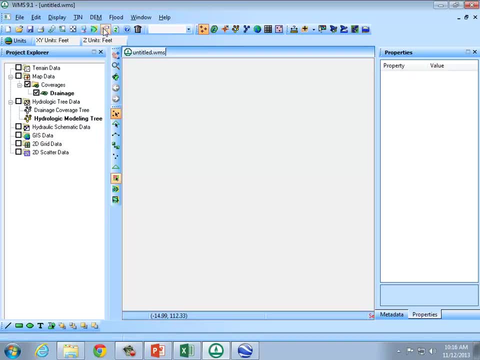 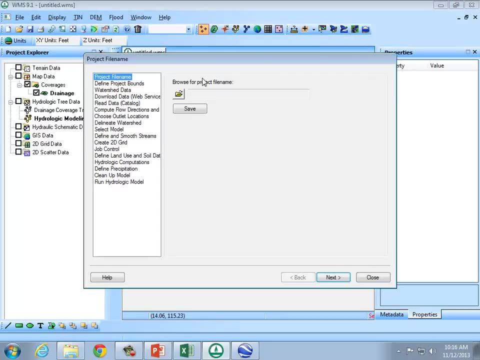 go forward in the view and so on. So I'll just sort of introduce the rest of the buttons as we use them along the way. Let's start up the hydrologic modeling wizard. The first thing you do in any project is create a file name that you're going to save it to. 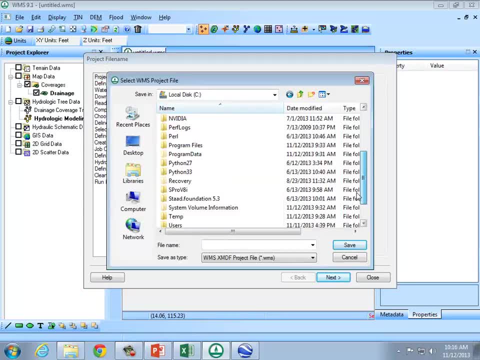 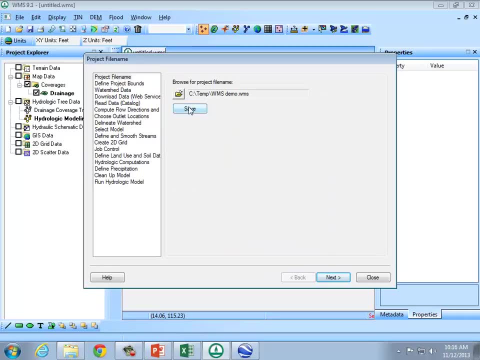 So I'll just go to sort of a temporary directory here and I'll call it WMS demo And you actually have to click save or else it won't save the file. You notice up here it still says untitled until we click save, and now it's actually established that file name. 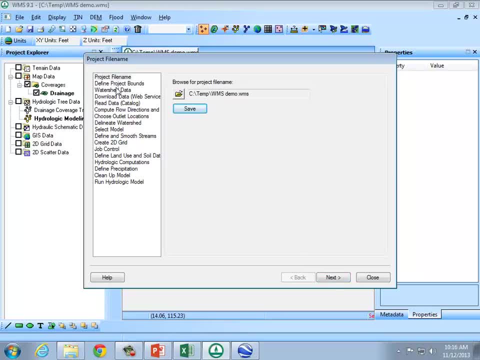 Click next to go through the next step in the workflow. So here is the overview of the workflow and we'll step through it back and forth. So next puts us in: define project bounds. Sometimes the hardest part of setting up a watershed is actually knowing where it is. 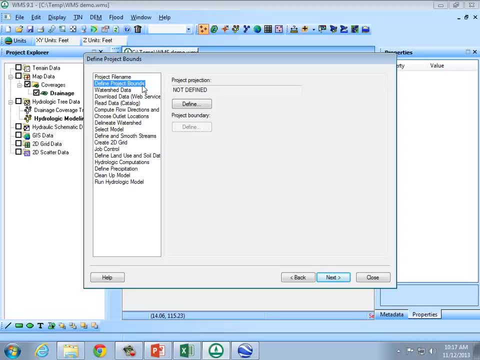 because you'll know an outlet or you'll know an area of interest, but you may not know precisely how far upstream the watershed goes. And especially in West Virginia, where we've got mountains and valleys that are curving in all directions, it can sometimes take three or four different tries. 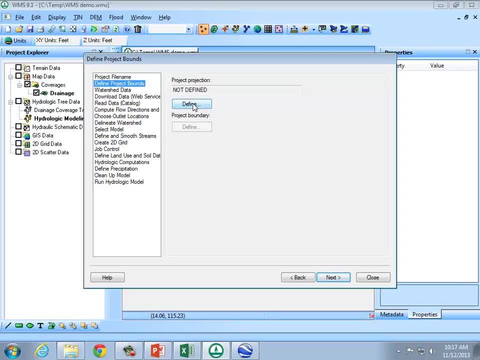 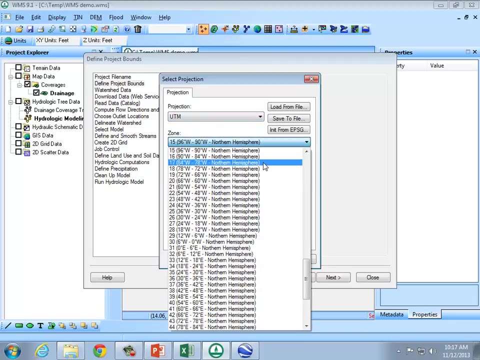 to finally be enclosing the entire area of a watershed. So you click on define to set up the project projection, and what we're going to use for most of the projects that we do is something that's called UTM Zone 17.. West Virginia is in UTM Zone 17.. 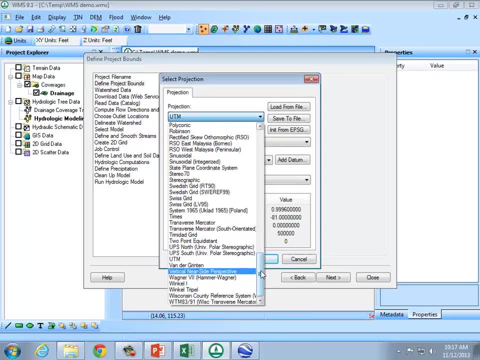 And not to get into too much of the boring details, but each one of these is a different way of keeping track of position on the earth And, for example, you know latitude and longitude that you get on a GPS. Lat long is one of these many different methods. 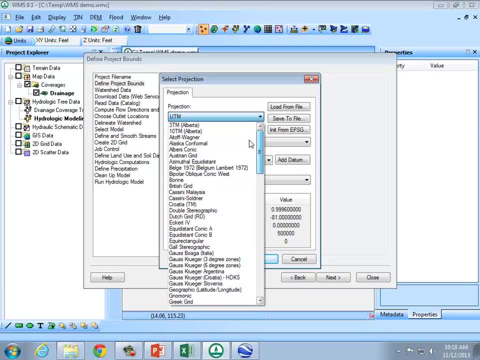 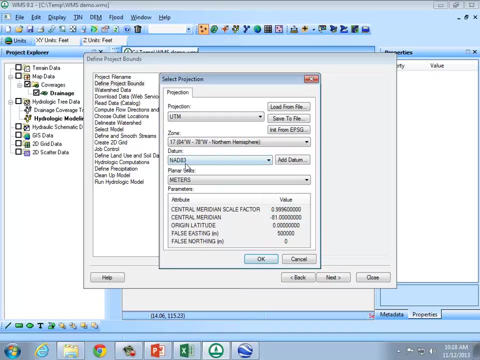 but UTM is the one that's very commonly used for GIS data at sort of like the state level. Sometimes we'll have to convert between the two, but we'll just start off by saying UTM, Zone 17,, which is what we have here in West Virginia. 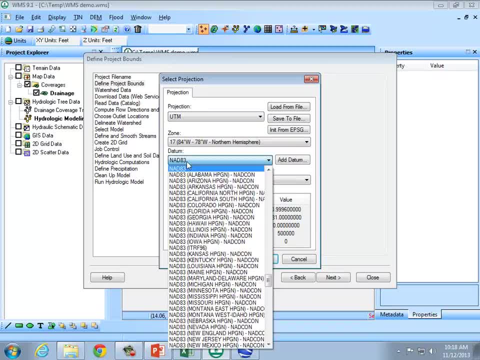 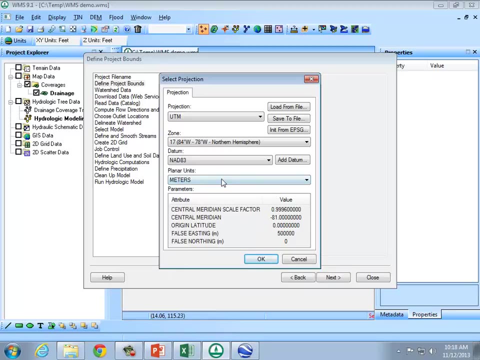 A datum has to do with what you're considering as the zero point for elevation and where you're fixing your your back and forth measurements, And you can see that there's really a lot of them as well. We'll just use a NAD 83 without specifying any particular state. 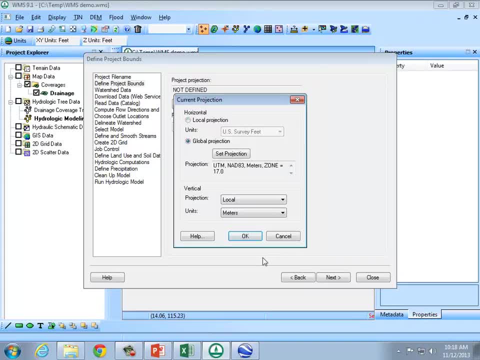 and units of meters. Sometimes you'll get a warning message that you need to to convert into a projected coordinate system and you just always pick UTM, Zone 17 and that'll be fine. A projection NAVD 88, that's a vertical datum. 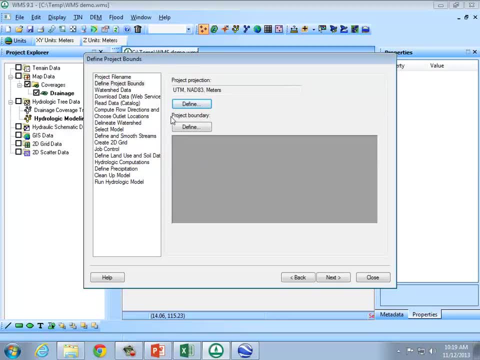 If you get into a graduate level GIS class, you can worry about all the, all those fine points. So we know the projection. Now it gives us the option. previously this was grayed out. Now we can pick the boundary and it pulls up a special tool. 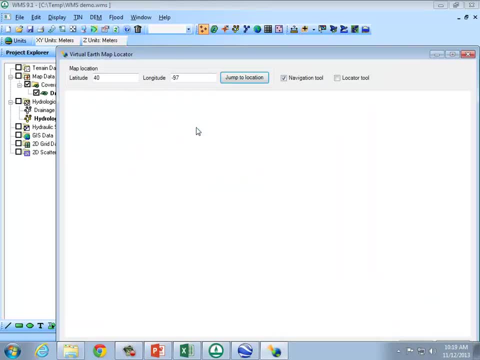 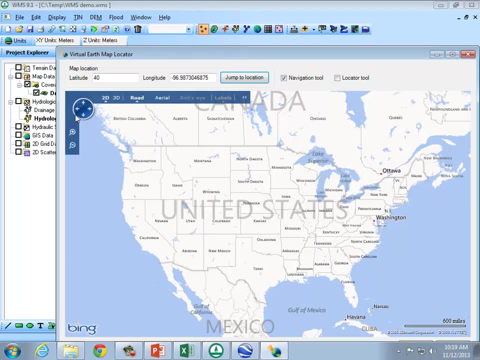 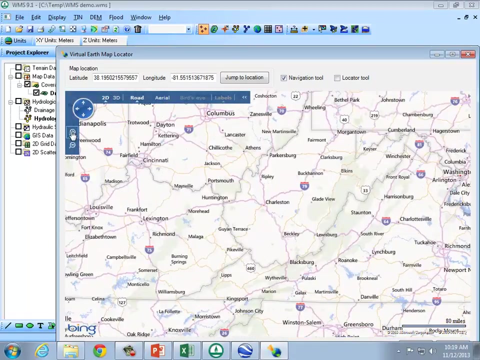 that brings up a map that streams to WMS. It's sort of like, I think, based on Microsoft data. You can see Bing down here. That's the giveaway. You can zoom in using these tools here. So we'll find West Virginia and we'll zoom in on an area of interest. 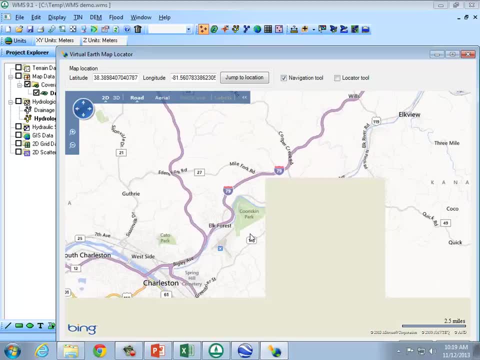 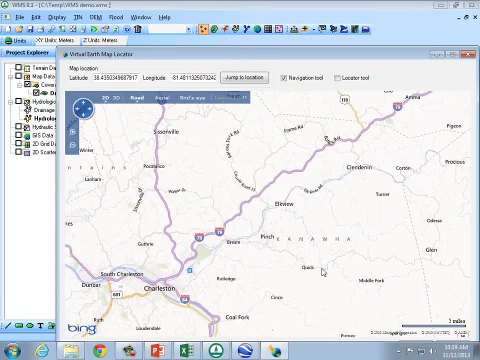 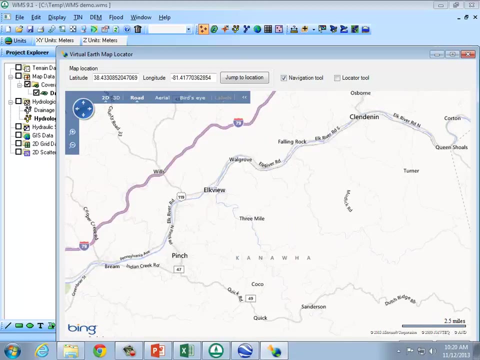 Ah, there's Charleston. alright, There's a watershed I'm acquainted with in Charleston, sort of towards Clendenin. Yeah, in this area, Alright, So let's say that you're interested in where this stream crosses a particular road. 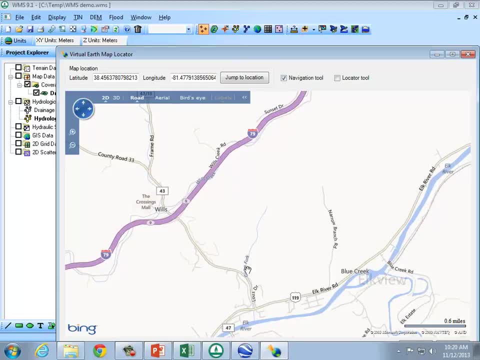 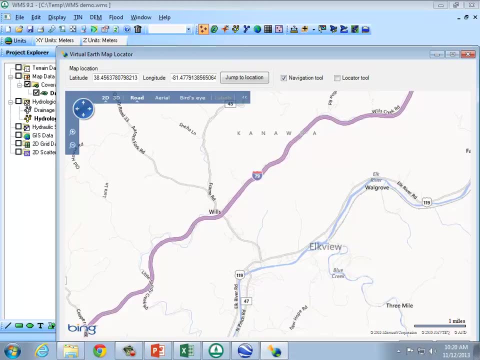 It looks like this is 43, given fork. There's a stream there, So we know there's a watershed. but what I was saying, how this is sometimes an iterative process, it's not yet showing us any of the ridge lines, And so you don't want to have it too far out. 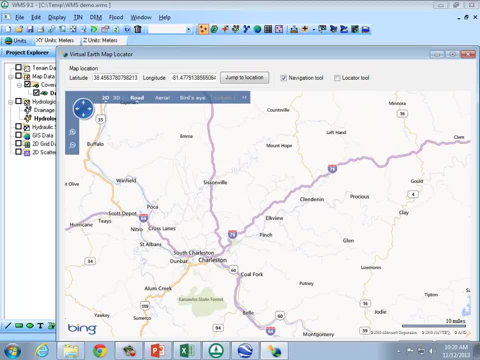 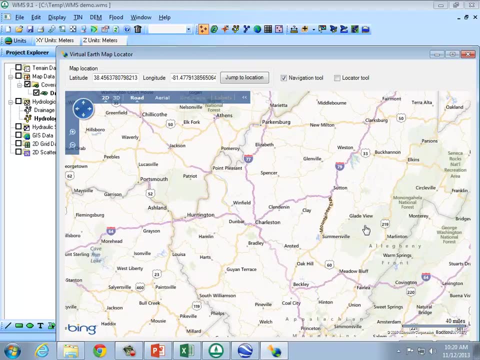 Like if right now we most certainly have the entire watershed included in the project area, but if you have it zoomed out really far, you're going to download so much elevation data. it's going to have a huge file size. it's going to take forever to get the data. 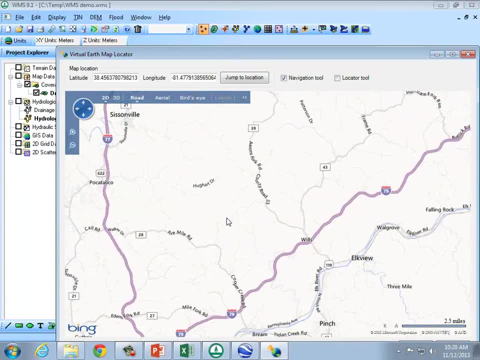 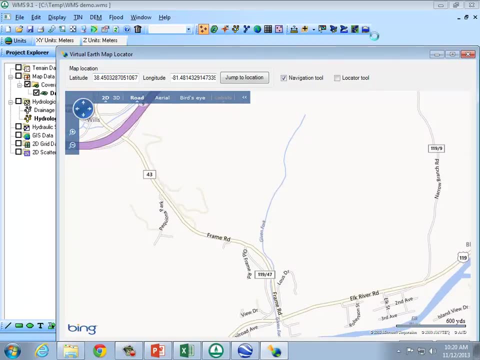 So you want to narrow in on it as much as possible, but you don't want to zoom in too much, because if you zoom in too much then there's a chance that right now the ridge lines are outside of the project area. So let's actually zoom in too close. just to give you an idea. 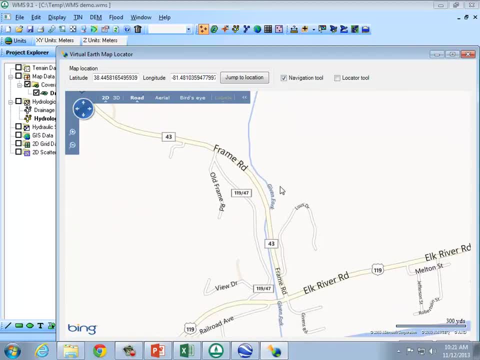 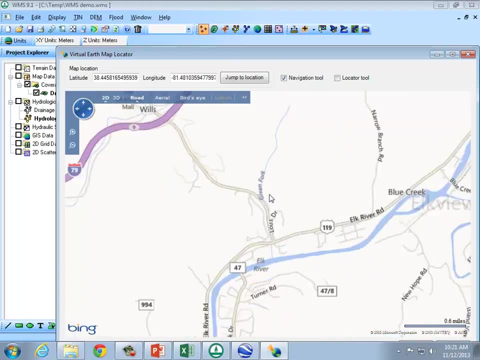 If I want to delineate this stream as it crosses the road, so like I'm putting in a culvert in this road and I want to know how big should the culvert be? Alright, so I've got the whole stream and I think maybe this is all of my project area. 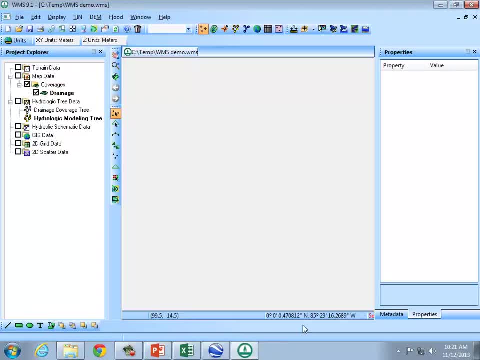 then I can click OK, But deep down inside I sort of know that that's not going to be the right thing. The wizard went away. it's not visible right now. that's just sort of a small little program bug If you just click right here on the tool. 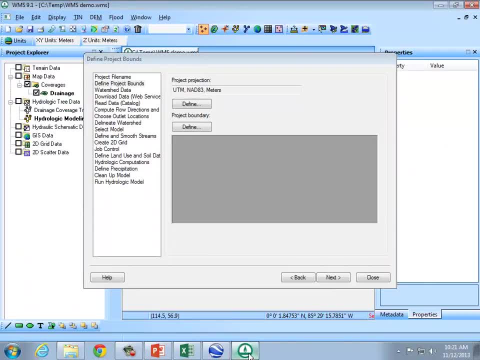 it'll come back up again. It has little idiosyncrasies, little ethnicities like this, because this software is actually written by students. The programmers for it are masters and PhD students at a university, so it's a great program. 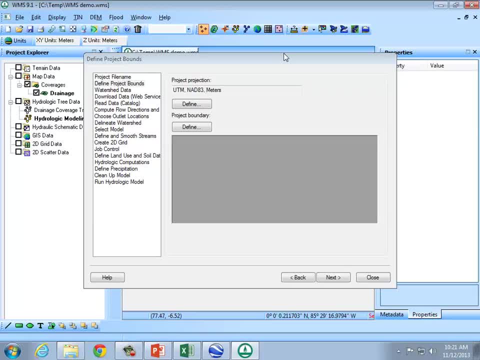 but it's not polished to the same level that maybe an operating system would, or a product with big commercial backers. So we've got the boundary defined there. If I go back now, it shows me the coordinates. That's another thing. I wasn't able to actually see the coordinates. 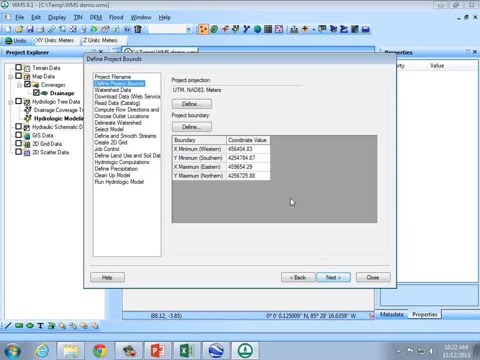 until I went back and forth here in the workflow. So these coordinates, it's just basically drawing a rectangle. You see it's got the four corners defined and these coordinate values. it's not like latitude and longitude where you have degrees, minutes and seconds. 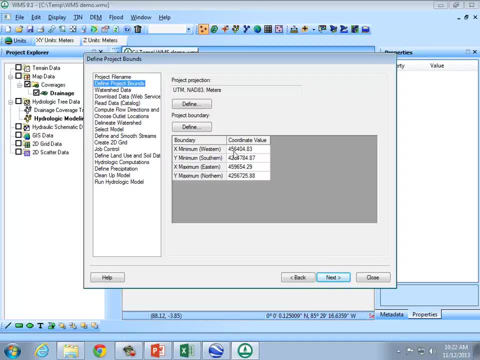 Each one of these is a meter, and so you can trace your cursor over the screen and it will tell you either the lat long or it will tell you the UTM coordinates. So the next thing it wants to know about is where should it go to get the data for the watershed? 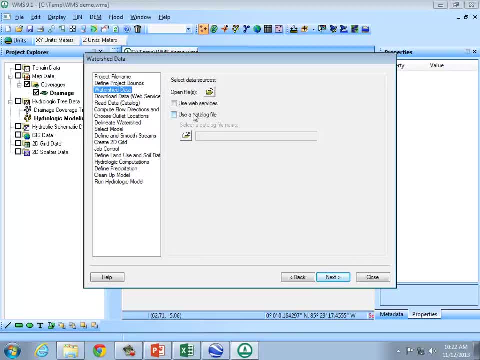 And you can either have it open your own data files or go online- the so-called web services- to get the data, And the main three data points that we need it to get are elevation data, soil data and land use data. So I'm going to click use web services. 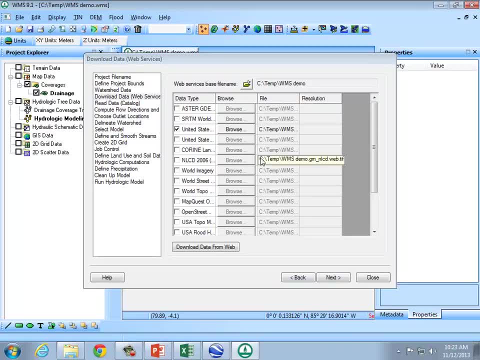 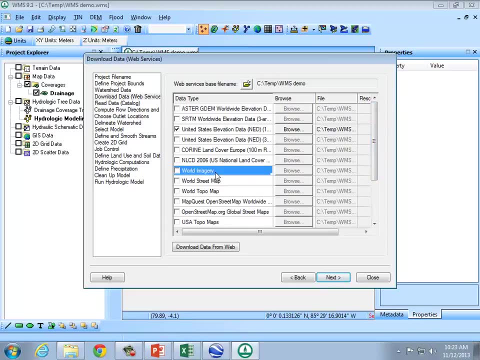 and have it, give me the list of what data is available. Here's a whole bunch of different types of data it can go and get. It can get images, for example, a street map, a topo map, like maybe if you've gone camping or hiking before. 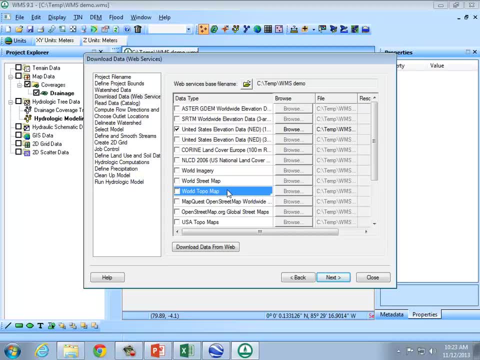 you have a sense for what a topo map looks like. Usually it has like contours and it shows streams and campsites and so on, What we'll ordinarily be interested in. I won't add the maps this way, but I'll ask it to go get DEM data, so elevation data. 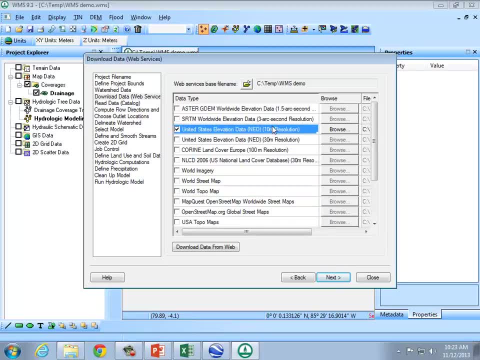 And you can see that there's two main options here: 10 meter resolution data and 30 meter resolution data. That's talking about how far apart the pixels are. for the elevation data spacing, It's sort of like it's going to download a grid. 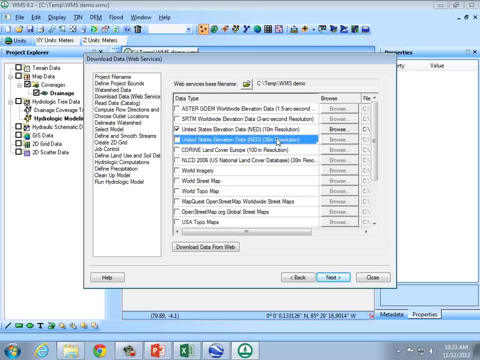 you know, we have a box that we've enclosed, and so I need to tell it to either go get the elevation at 10 meter spacing or at 30 meter spacing, And one of those file sizes is going to be nine times bigger than the other. 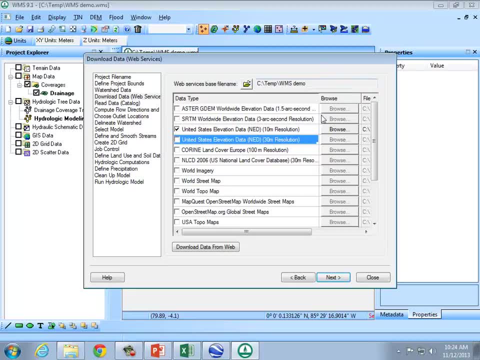 because 30 meter resolution. that's saying that you're going 30 meters this way and 30 meters that way, so there's going to be one-ninth as many pixels If you've got a relatively small area- 10 meter resolution. 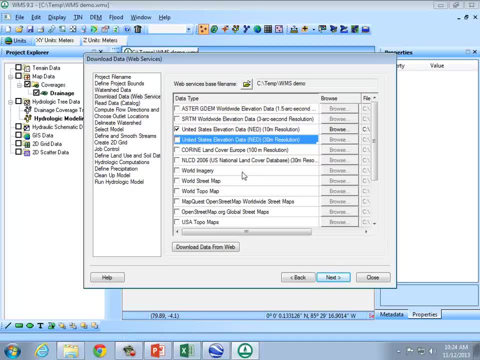 is what you should go for If you've got a big watershed- 30 or maybe even greater. So I'm going to tell it to get the 10 meter resolution data NLCD. that's the land cover, and I think they've just recently added the soil data. 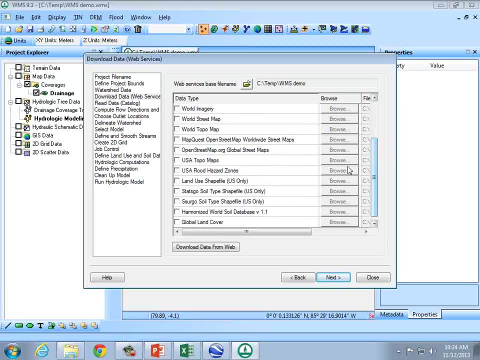 Previously it had to be added externally. We'll try it out, but it may not work and we want to get Sergo. We'll talk about the difference between Sergo and StatsGo. All right, so I click download data and it goes through this process of connecting to the servers. 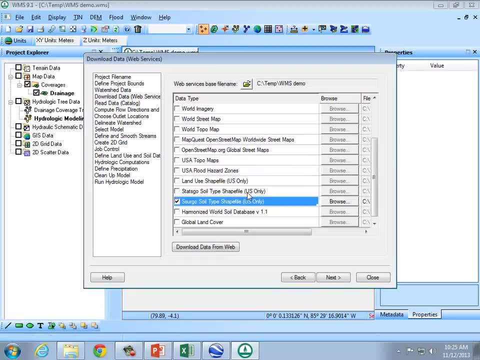 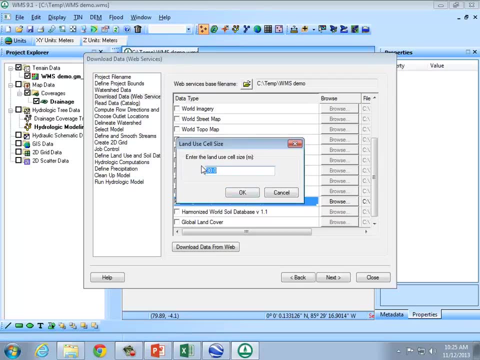 and getting the data. It wants me to confirm that this is a 10 meter DEM. It starts downloading it Now. what it's asking about is the land use. That elevation has a. the land use data only has a maximum resolution of 30 meter cell size. 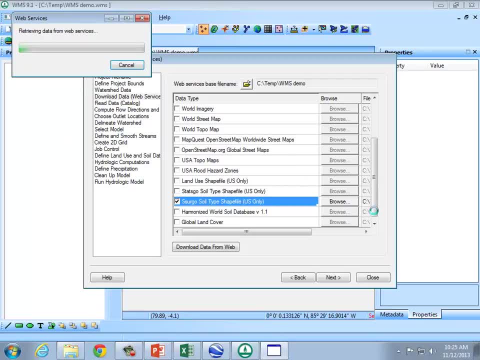 and so I just verify that. okay, and it downloads the land cover data. Now, the soil type is what I've sort of got my fingers crossed on. I haven't verified that it works. It's a relatively new feature they've added to go. 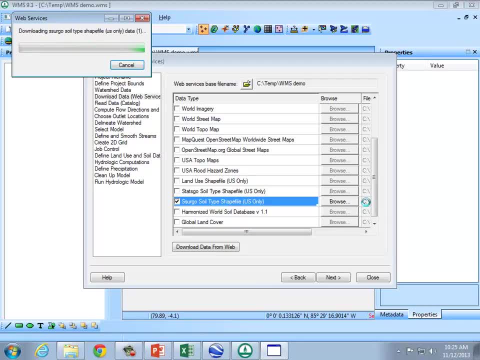 and get the soil data directly. Otherwise, I have a file of Kanawha County soil data that I can have it load in manually. if it doesn't get it automatically, I'll give it a minute and cancel it if it doesn't seem to be working. 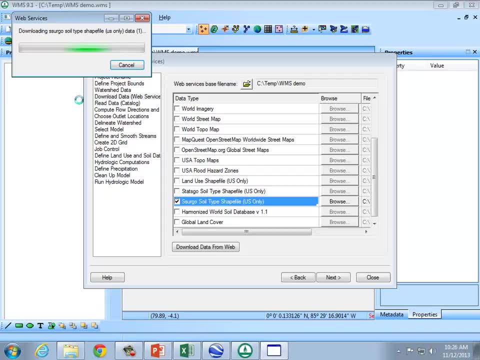 So why do you think, while it is working, what's the purpose of setting up a watershed model like this? I mean, besides the gee whiz factor of, you know, playing with fun software, what's the practicable purpose of doing something like this? 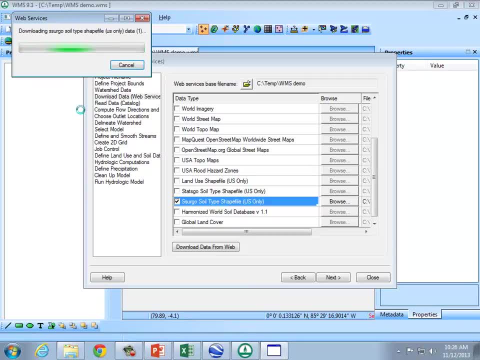 All right, find the peak flow rate. yeah, and why would we want to know the peak flow rate? Culvert design, pond design, stream design, channel. you know, like any of the hydraulic design that you need to do starts off with some flow capacity. 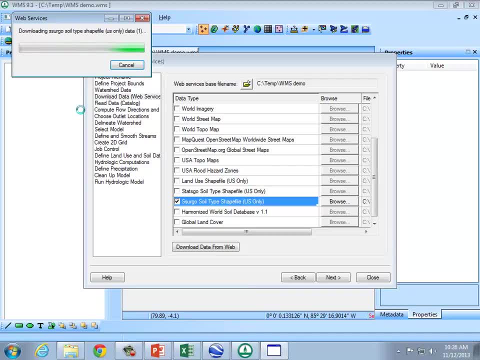 whether it's managing the locks and dams on the Ohio River or whether it's just designing a ditch for a farmer to irrigate fields. There's a flow rate that the channel has to carry, and this is a way of estimating what the flow rate's going to be. 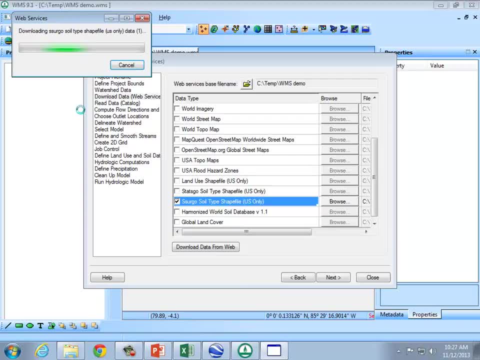 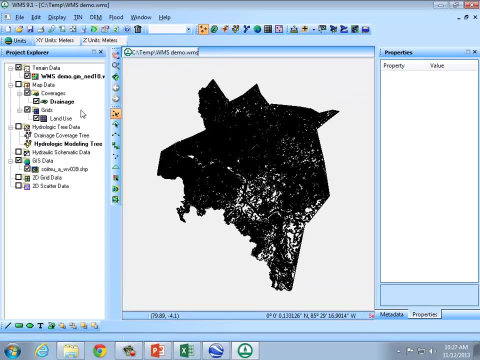 And it's really no better than an estimate. In hydrology, there's so many variables that- oh, it looks like it got it. Yeah, it did. There's so many variables that we have to be really honest when we're giving our answers. 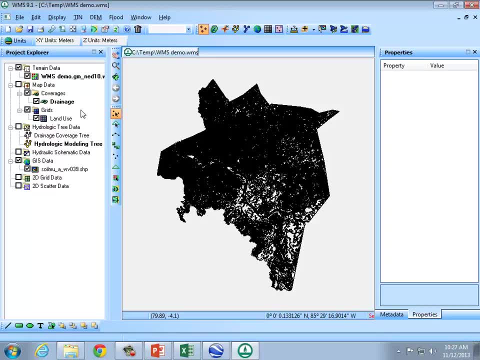 You know you can calculate that the peak flow rate is 1992 CFS per inch. but sometimes it also puts you at a disadvantage. So it's really it really pays to report what the confidence interval is. You know a confidence interval if you remember. 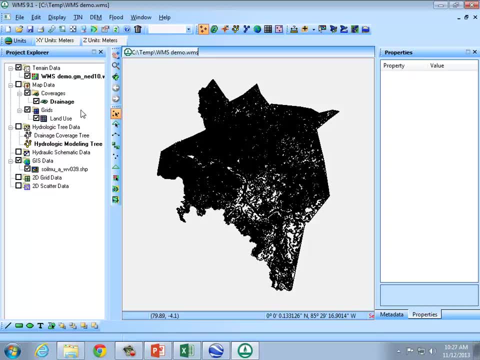 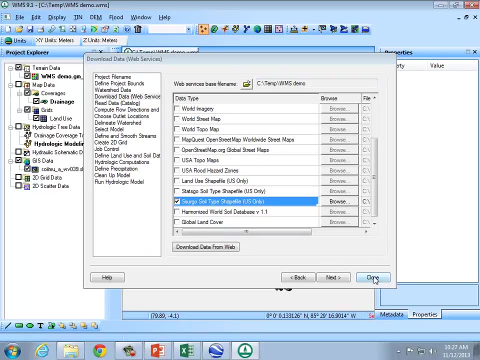 from your statistics class would be that range of flow rates that maybe you have a 95% probability that the actual value is within that range, and so, All right, we've got the data that we need. Now this wizard can be closed at any time. 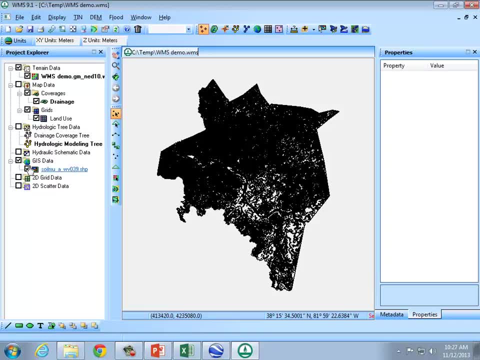 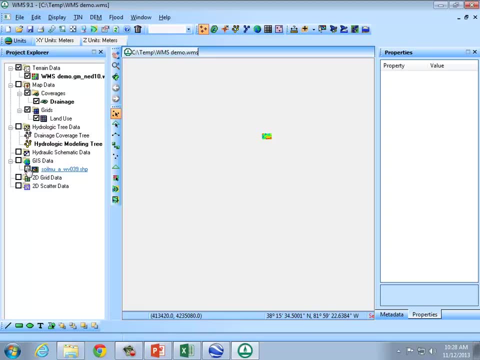 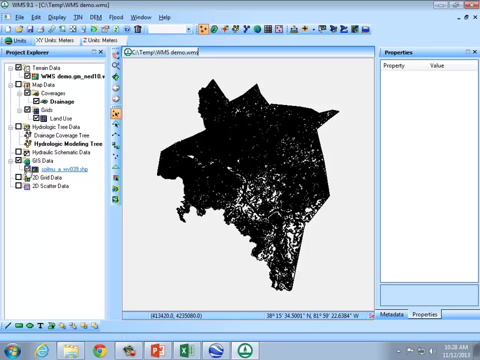 and you can open it again at what data it's given us Right here in the GIS data. that's the soil type data, So I'll turn it off because it's sort of making everything else really hard to see. There's our elevation data. The reason why it looks like that is it gave us the entire county. 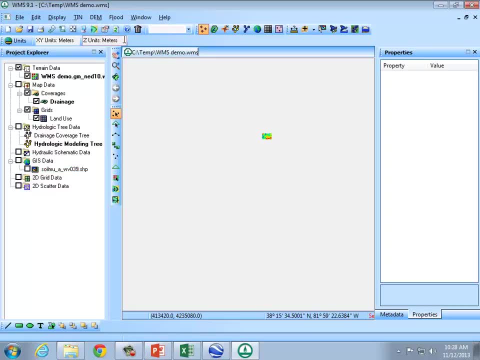 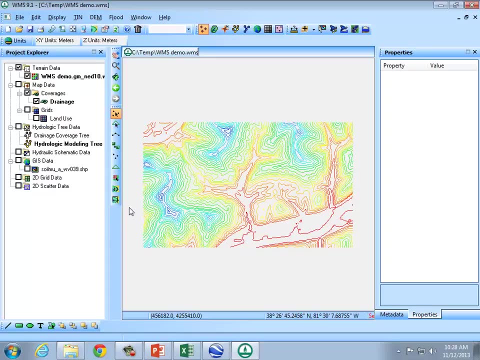 That's all of Kanawha County, So let's zoom in on. this is the area of interest. I'll turn off the land use grid for now. So these contour lines basically just show the elevation. Now let me bring in a map to refresh your memory of what we're looking at. We're looking 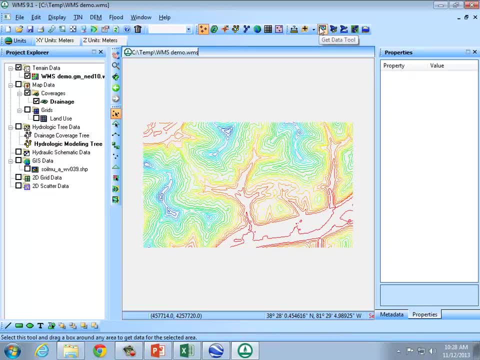 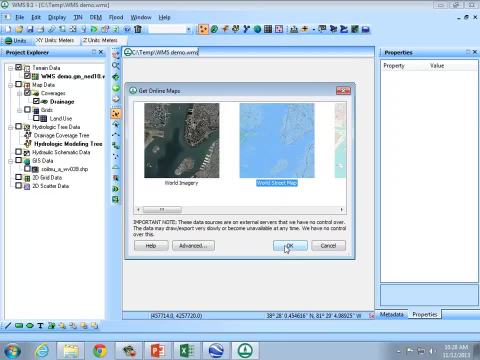 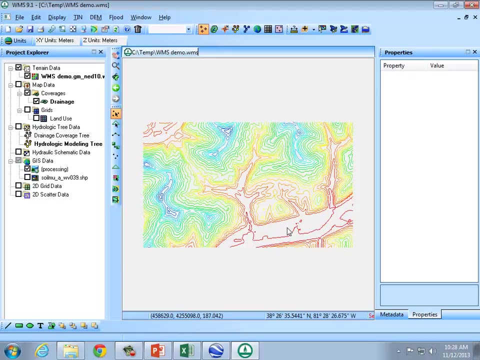 at a street and a stream that was crossing the street. So there's one of these: get online maps. There it is, And what I'll do is the world street map. It's usually really nice. It's got all the roads that we'll need and it sort of hints at the contours. These world 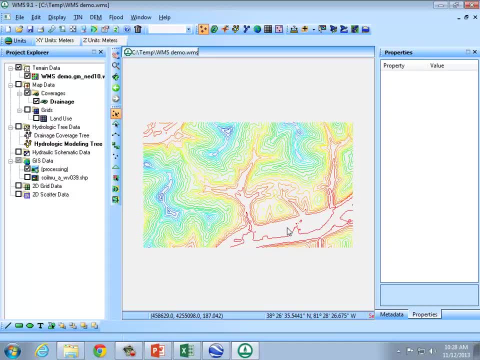 street maps are pretty useful for hydrology. I'm glad that they have access to them. You can see right here it says it's processing. It's just streaming that map, So anytime you zoom in it has to go through this processing procedure again, unless you make a static version of that, Like if you. 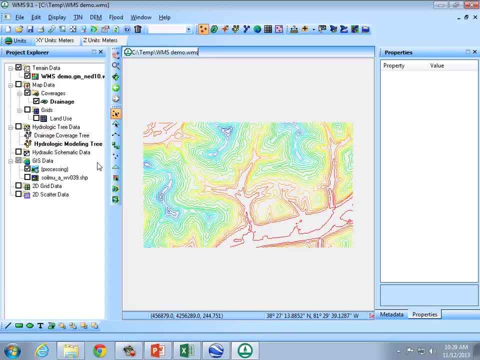 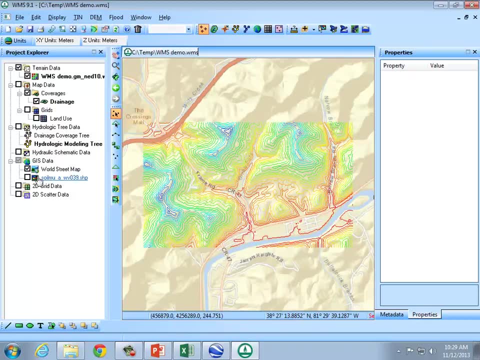 save it to your hard drive. then it won't have to go through the process any longer, And I'm sure when all of us are working simultaneously it'll probably bog the system down. There we go, So I'm going to save it, and so it doesn't have to stream anymore, If I right click on. 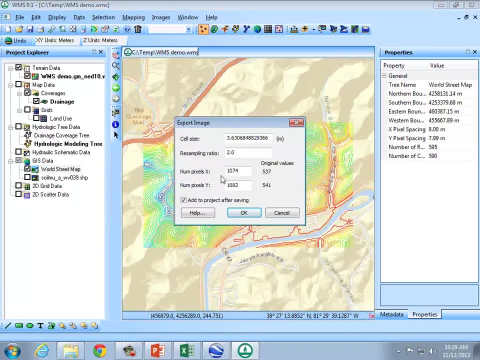 it, then I'm going to export that as an image, And this resampling ratio of 2 means that it's going to zoom in a little bit when it saves it, So I can have higher resolution even if I zoom in further. So I'll just leave. 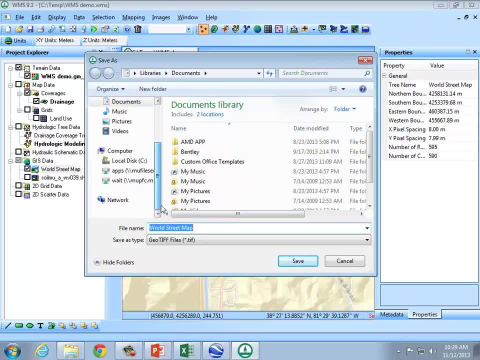 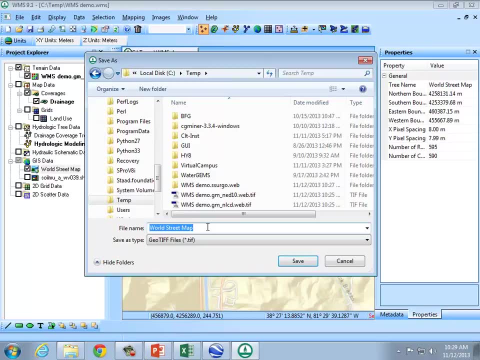 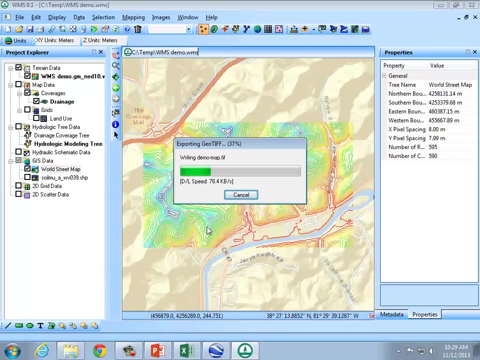 it at the default of 2 and click OK, And it wants to know where it should save that map that it's going to create. So I'm going to call it Demo Map. This TIFF file is georeferenced, which means it's going to save the map that it is going to create, that it's going to Samuel. 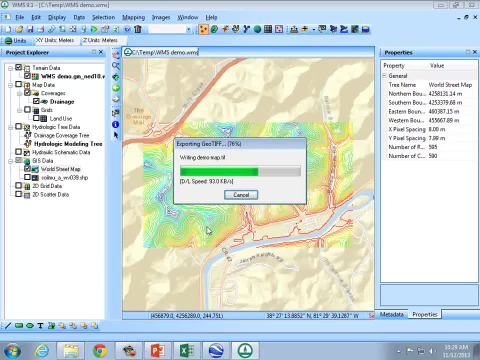 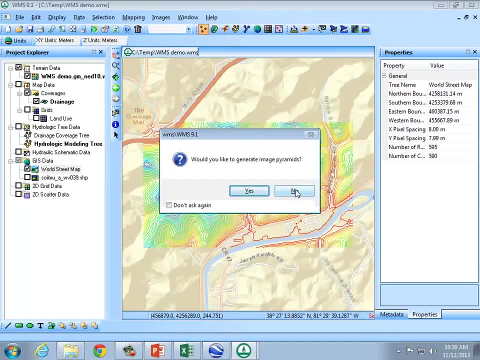 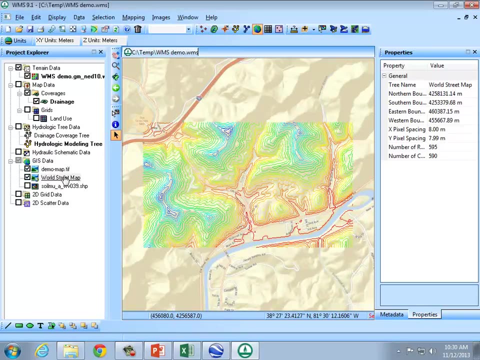 It's more than just an image. It also has coordinates that defines where the corners are, so that if you open it up in a program like this or another GIS program, the image is placed on the screen where it needs to be. So let me turn off now this one that would be streamed. 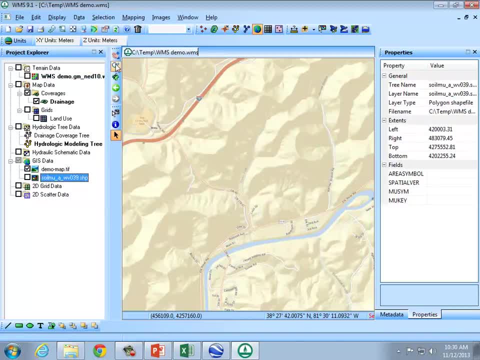 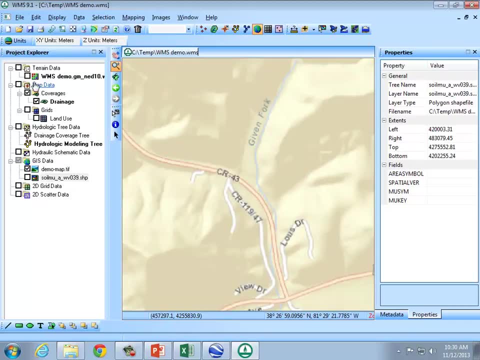 and I'll turn off the contour lines and we'll zoom in. Remember what we are curious in is this given fork crossing the road there, So I can turn on the contours and see that they sort of match up with what that image is implying. 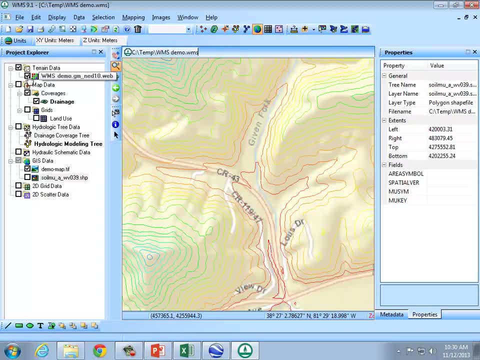 It's showing that there's a ridge line there. What do ridge lines look like? on a contour map You can see that here's the top of the. from the shading we can tell that there's the top of an area. Zoom out a little bit. 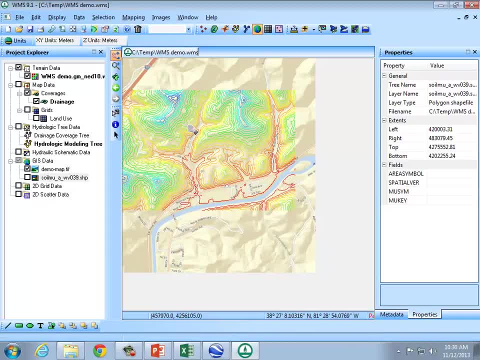 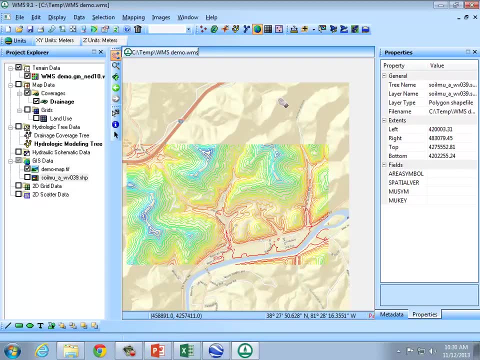 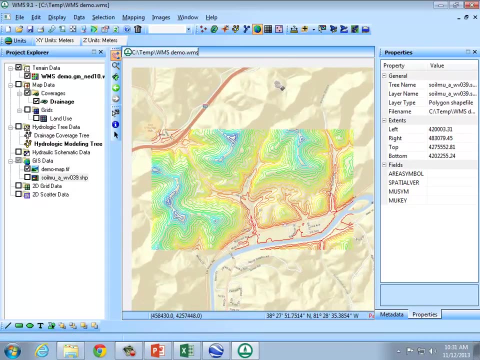 But remember how I said, deep down inside, I sort of suspected I didn't have all of the area that I needed. It looks like I don't have the entire watershed, And so the way I can confirm that for sure if I go back to the modeling wizard- 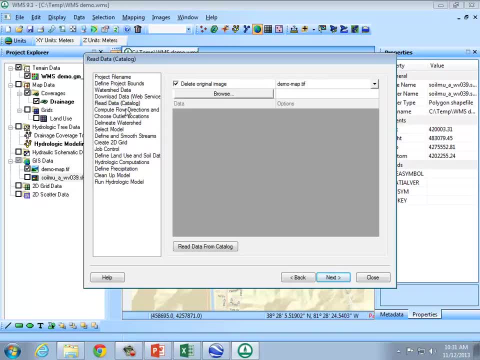 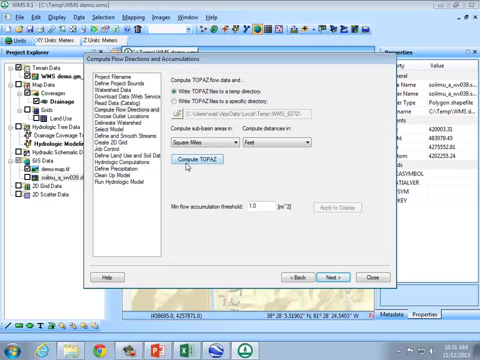 we were at download data. We did that. It already read in the data. Okay, compute flow directions. There's this program called Topaz, and what Topaz does is it compares all the cells and trajectories. It tries to figure out where water is flowing to. 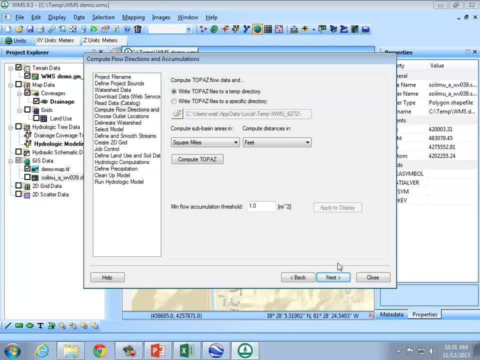 What's the relationship? You know, if water falls in one cell, will it go to the left, right, up or down? It just looks for every cell at which of the adjacent cells is lowest And from that comparison it knows. by doing it. 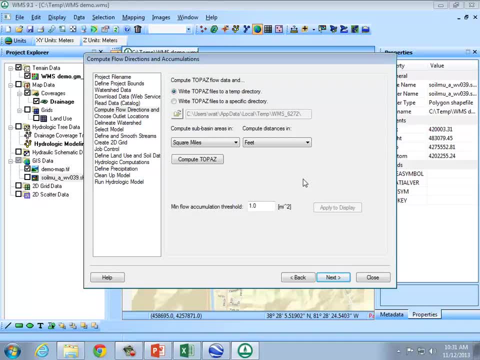 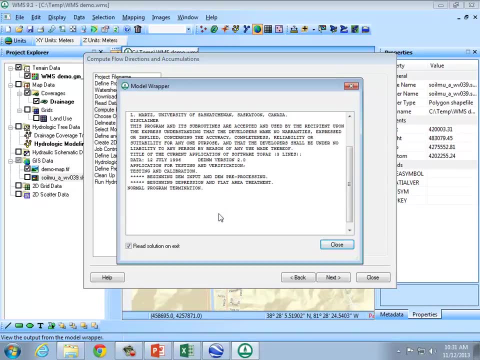 to every single pixel in the DEM network. it knows what way water will flow. So I just click compute Topaz and it starts and very quickly will finish And It will start to show where the low flow area, like where the streams, are likely to be in our map. 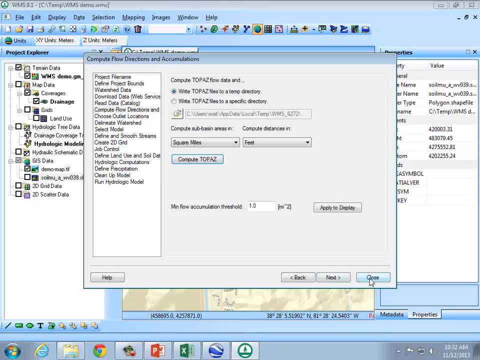 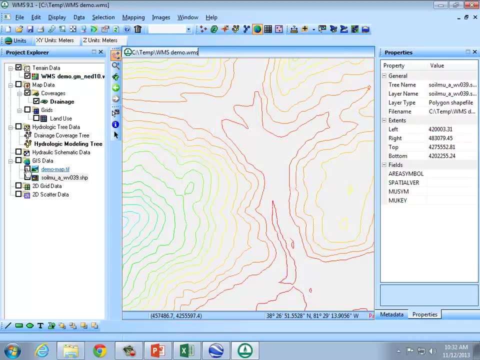 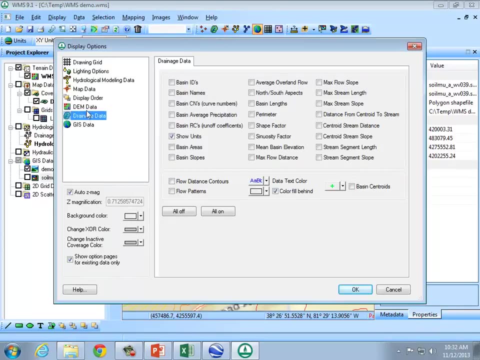 Oh, normal program termination. It's done All right, So I can close that and zoom in on the area here. It's not displaying them. The streams aren't turned on. Let's see if I can switch them on. Oh yeah, I better know what it is. 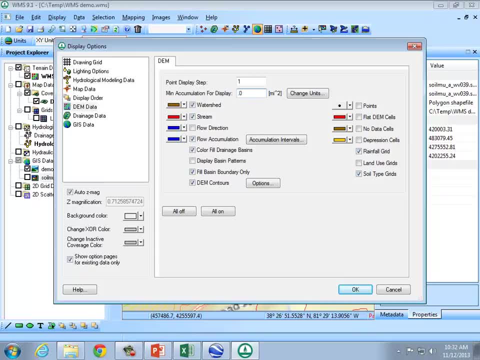 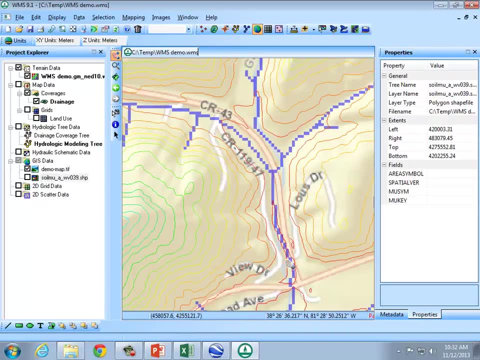 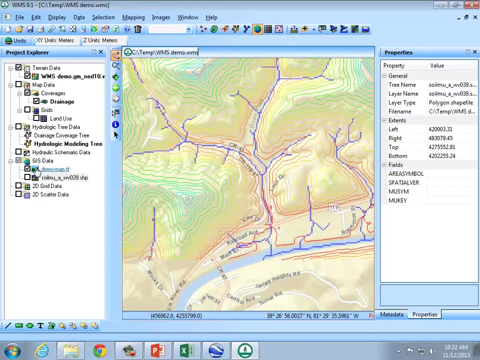 Here we have to decrease the watershed area upstream. that will lead to it. All right, there we go. So here it doesn't know from like the program can't see that there's that blue line from the image. It's just the. it calculated these blue lines based. 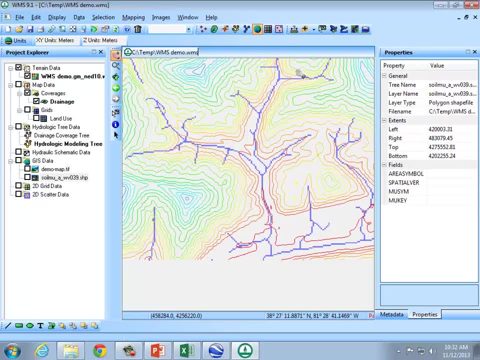 on where's the lowest elevation in a certain area, And so it's predicting that a stream will form there, because it has. It's a low point in the map, And so I'll pick out my point that I'm interested in. Remember it's that crossing location right here. 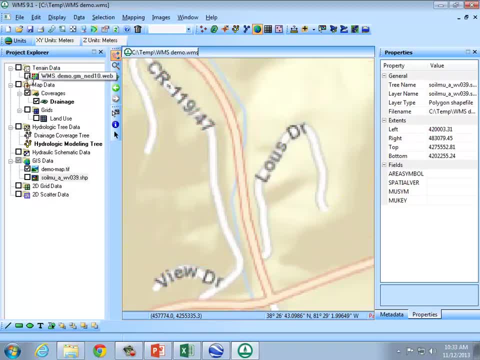 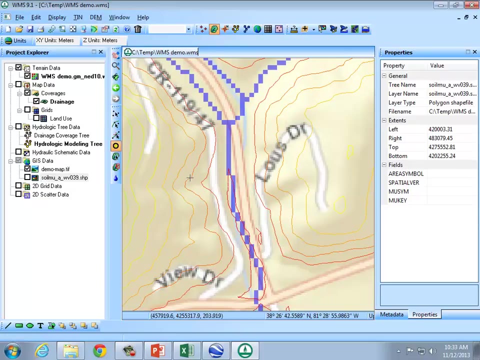 where the stream goes under the road, So the equivalent of that. it looks like there's a junction of sorts and then it goes under the road. So I'm going to put my outlet, Create an outlet point right there And, if we go back to the wizard we were at, choose outlet. 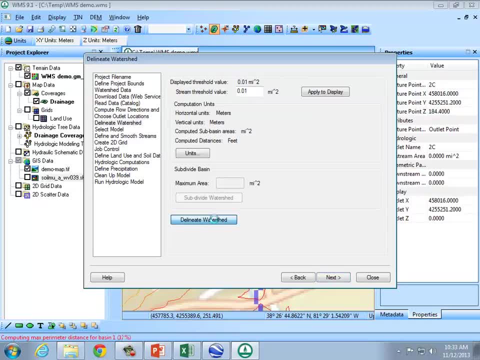 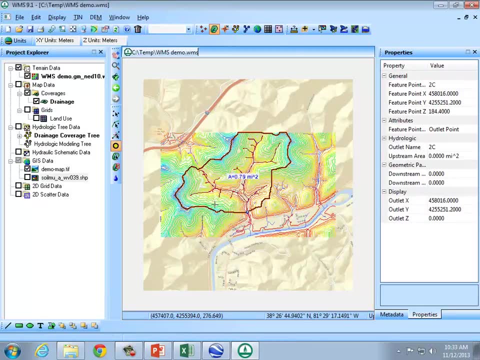 All right, we put the outlet down Now delineate watershed. So if you click this button delineate watershed, it'll draw a circle around your watershed area And you can see that it's seeming pretty regular And you know this is the way it ought to be. 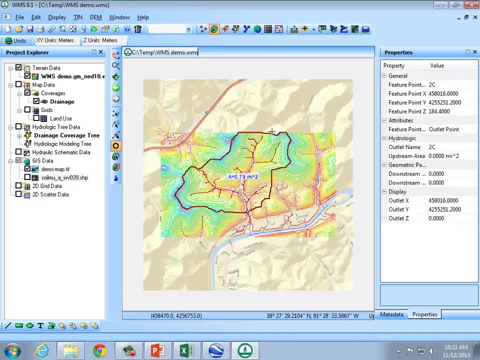 But then it's just all of a sudden, this flat line. That means I didn't capture the entire watershed boundary, So I have to go all the way back to the beginning, you know, back to the drawing board. So that's why it's important to try and do your best. 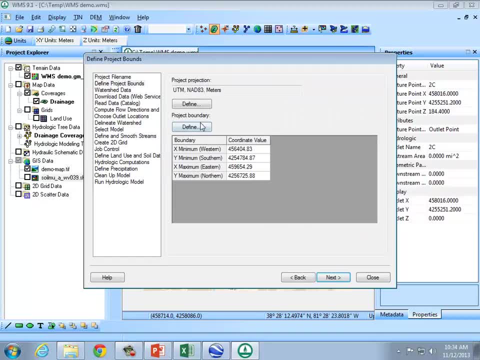 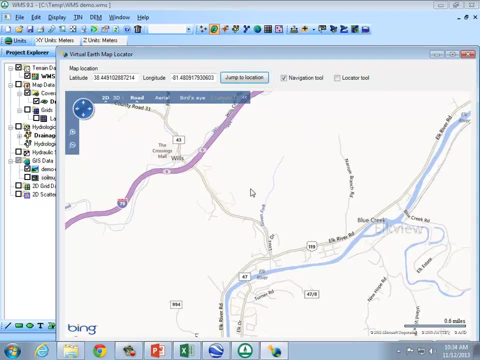 to delineate the entire watershed area. So I have to define my project bound, starting over with that. I can do it quicker than I did the first time, So we'll just pan down a little bit. We'll zoom out a touch. That's almost certainly in there. 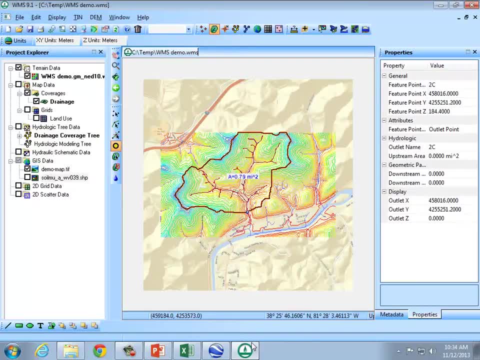 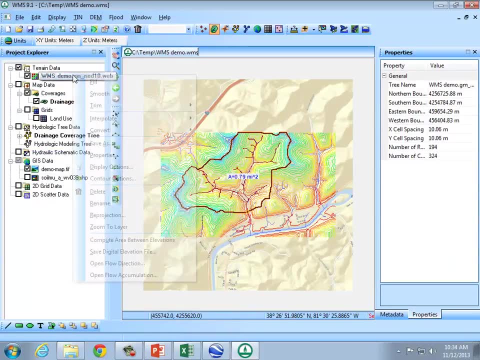 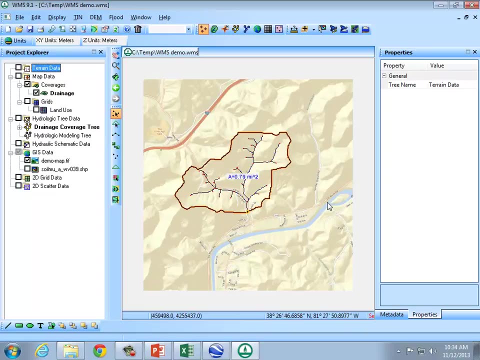 It took a while to download all that DEM though, all that DEM data. So this time, before I do that, I'm going to delete this DEM. All right, So back to the wizard, the wonderful wizard, The data we're going to get this time. 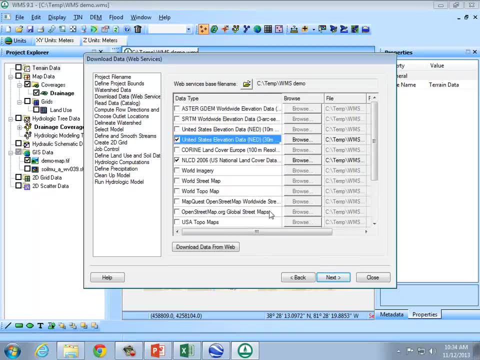 I'm going to have it get the 30 meter resolution data because it's faster And I already have this. I don't know, I don't need it. I already have the soil data still, so I don't need it. So it'll go and get the DEM data, hopefully quickly. 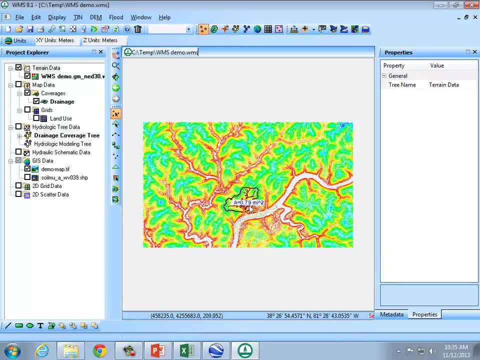 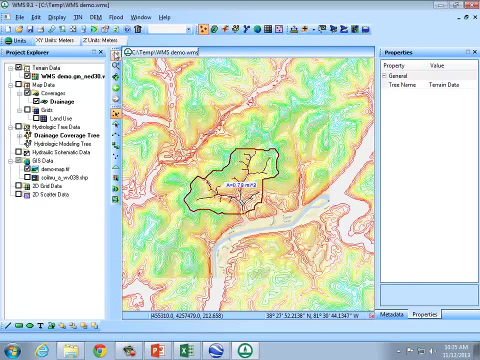 All right, Now I've got my watershed has got to be in there. I have to run Topaz again. So if I go back to now, all these things that are in the wizard are also in normal menu locations, And so when I'm in the drainage, 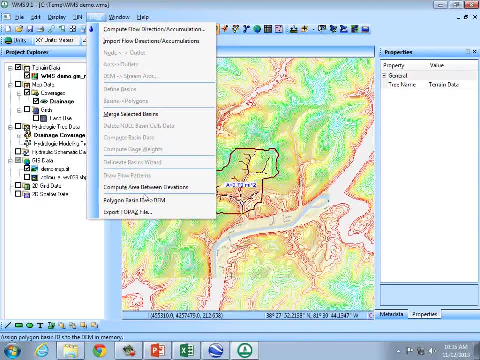 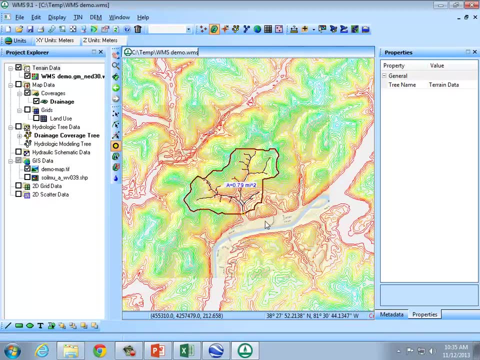 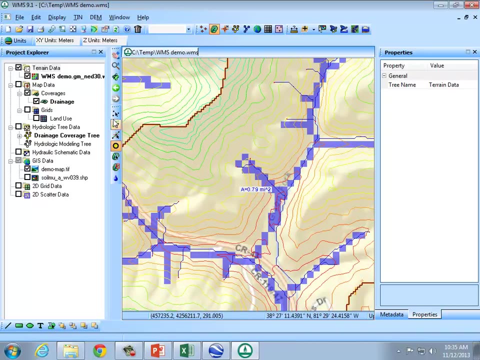 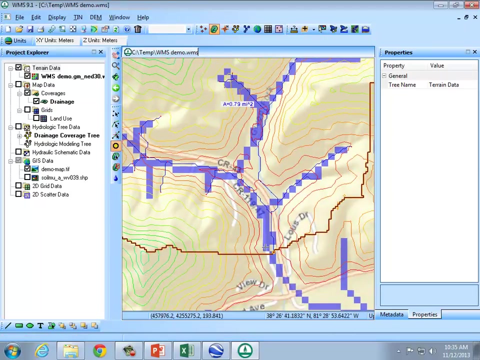 the drainage module. I can do Topaz, compute flow direction. That's Topaz, So it'll run it. There's all the streams And I'm going to put in an outlet again. Drop it there and delineate the basin. 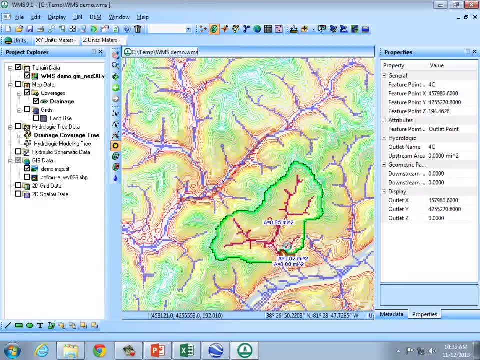 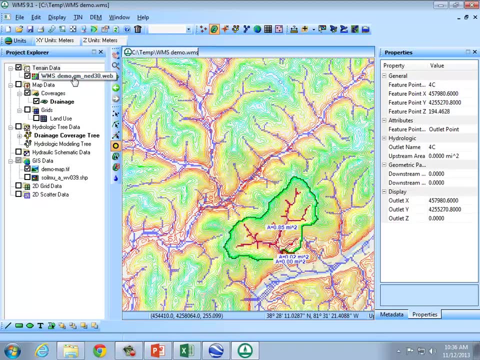 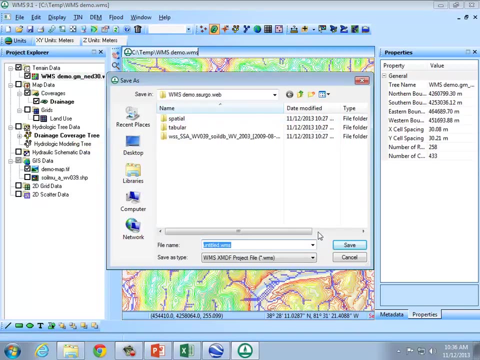 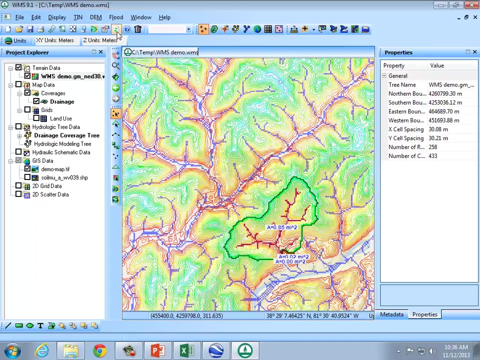 All right. So now it's got the entire watershed area shown, There's a way to export the DEM So you can save it. if you want to save pieces instead of the entire WMS file, like I'll save- And right now saving the dot WMS file will include the DEM. 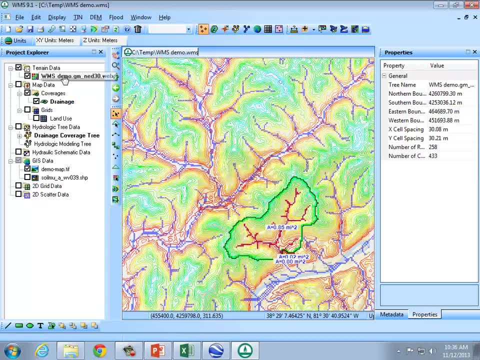 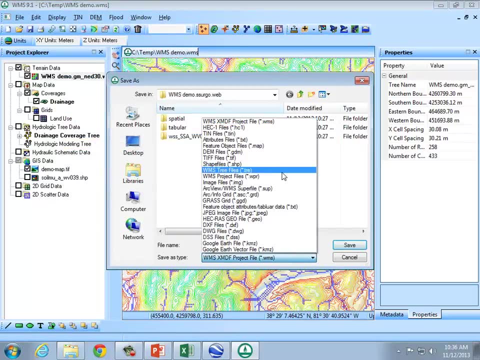 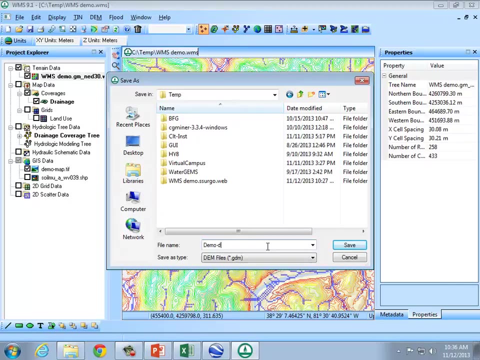 the drainage coverage, All the supporting data that I need, But if I want, I can save only the elevation map. It has many different file extensions that allows you to save, And so a DEM file. I'm going to just save the demo DEM. 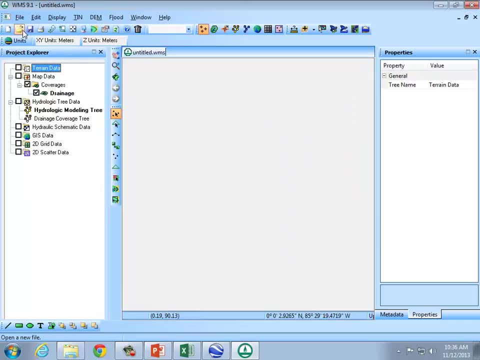 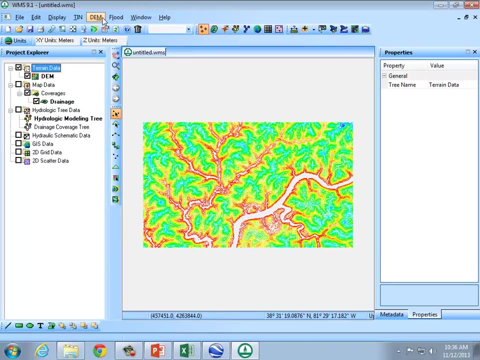 and then show you if I start over from scratch. I can open up that demo DEM file without having to go online, And I'm going to save it. I'm going to save it. I'm going to save it, I'm going to find it again and download it. 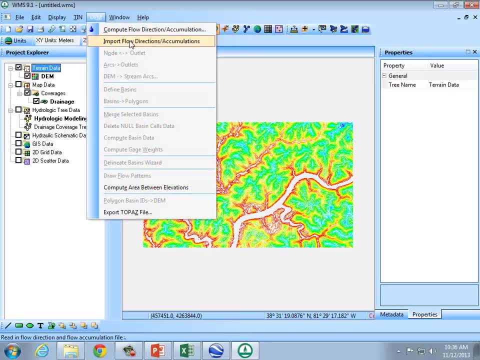 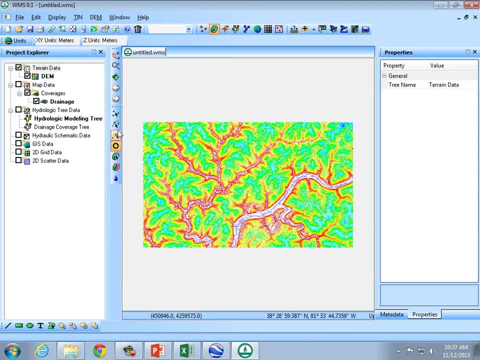 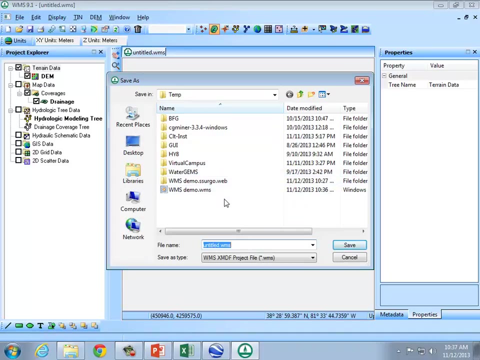 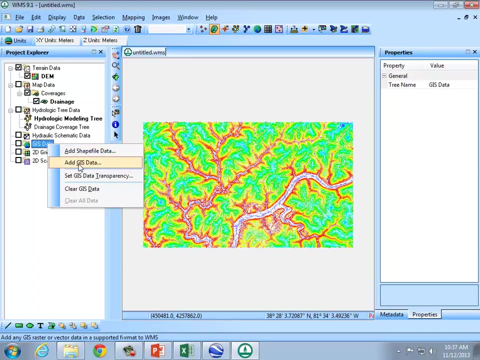 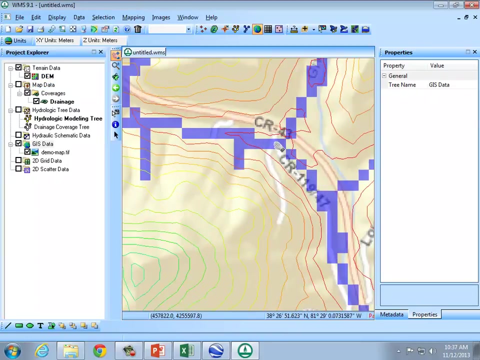 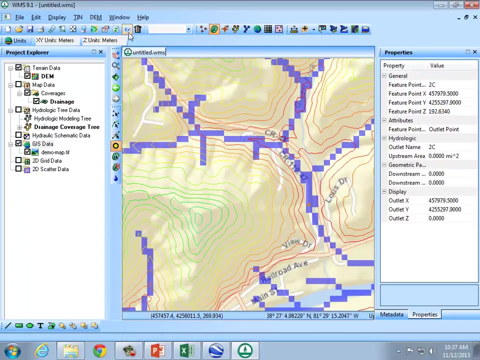 Okay, So run Topaz. It gives me the streams. I'm going to open up that image. Hmm, I thought I had an image here. Oh wait, maybe I want to. Okay, So I'll put in the outlet. delineate it again. 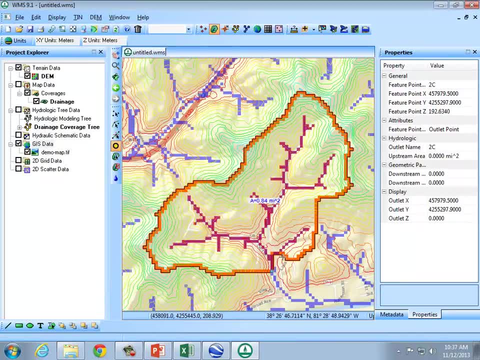 All right. So there's the watershed. Now we've got the boundaries of the watershed. Like I was mentioning before, The three main pieces of this are the elevation, the soil type and the land use. If I have it, go get the soil type and the land use again. I'm starting with a different project area. 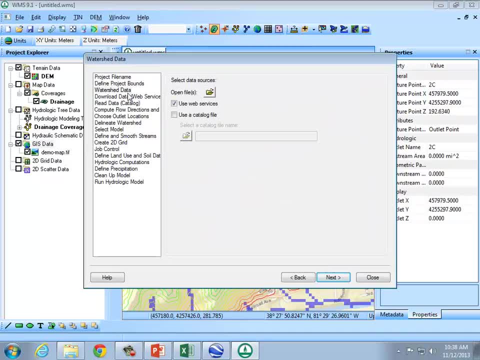 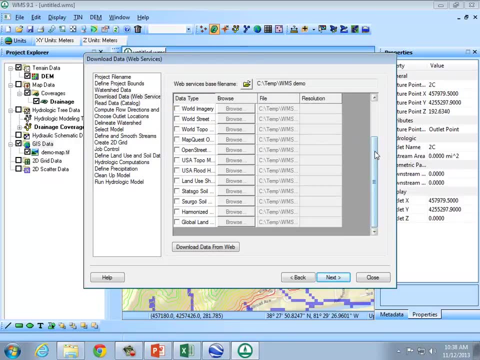 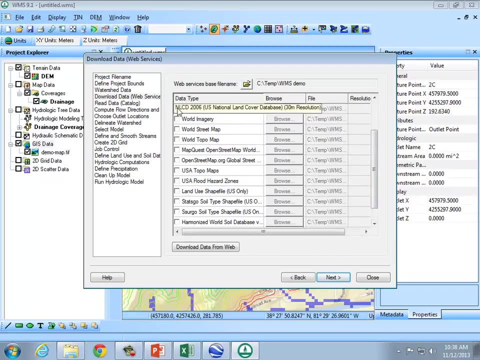 so I have to define. the bounds are still defined as the same and I don't need the elevation data. I do need it to get the land use and the soil type. Let's look at the land use stuff more specifically. Let me just focus in on that. I'll download it. 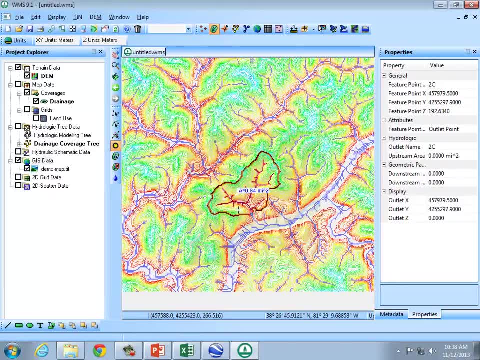 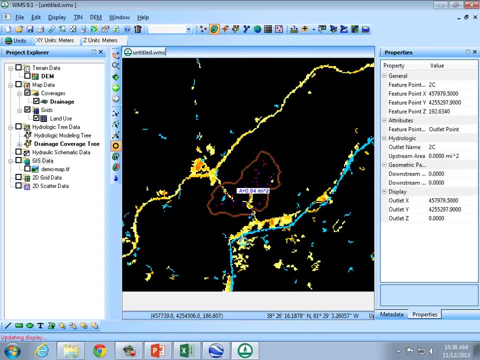 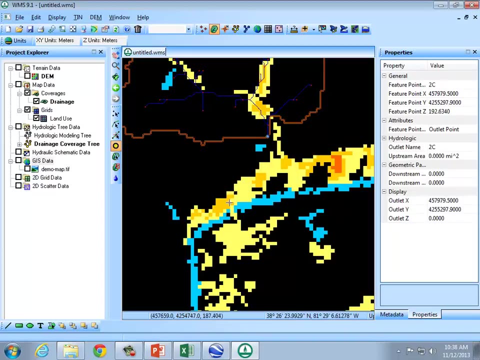 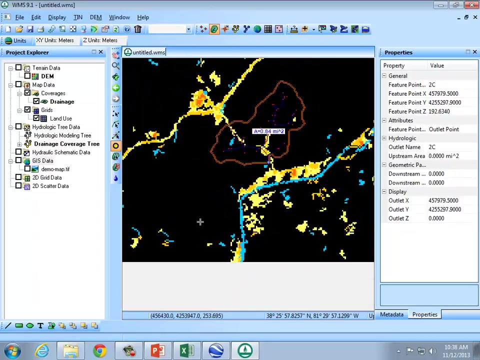 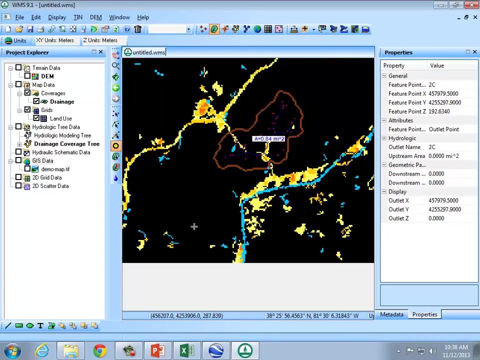 The different colors represent different land use. Here the blue represents water, What is indoor. Different shades of yellow represents urban areas. I think here black is being represented as a forest area. It's just telling you what they're doing with certain parts of the land. 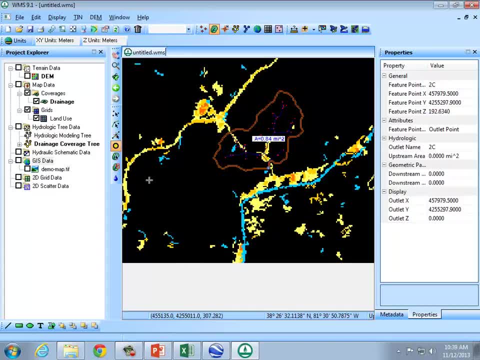 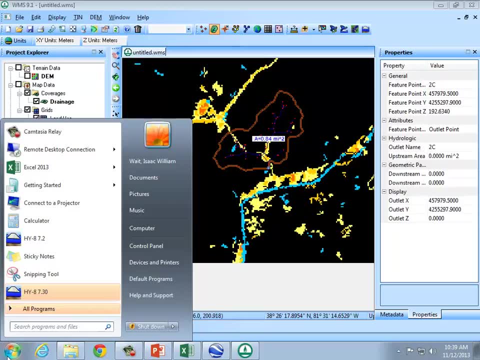 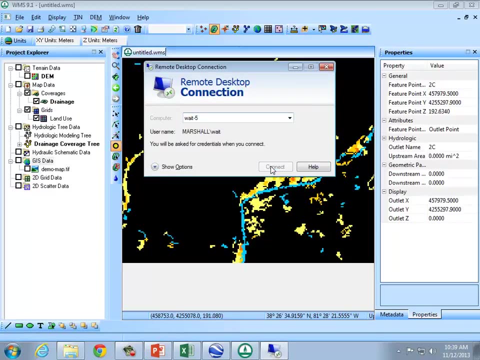 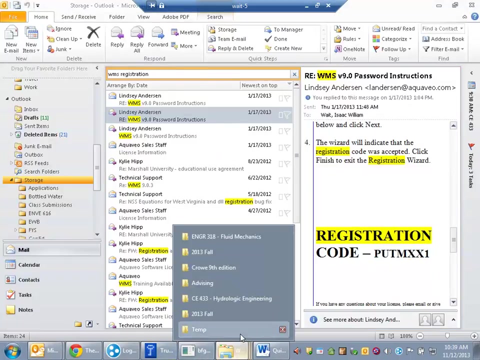 The underlying data. there is numbers associated. that comes with the land use code. Let me just quickly get the table that defines land use and it's how you map curve numbers is with this land use table and the underlying soil types. Just give me one second. I know right where it is. 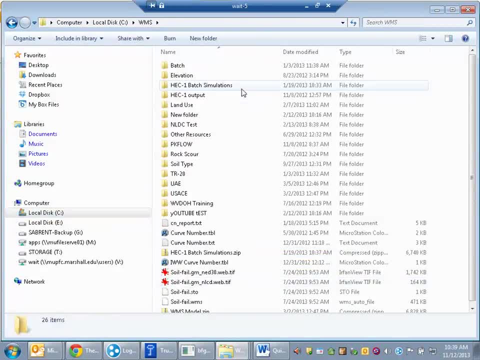 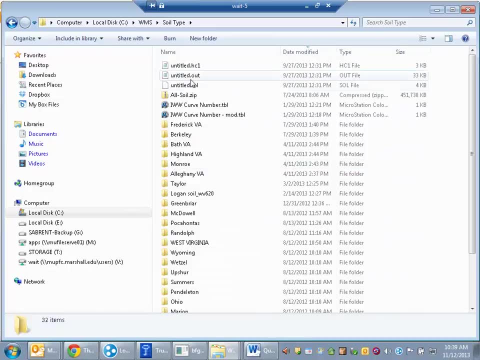 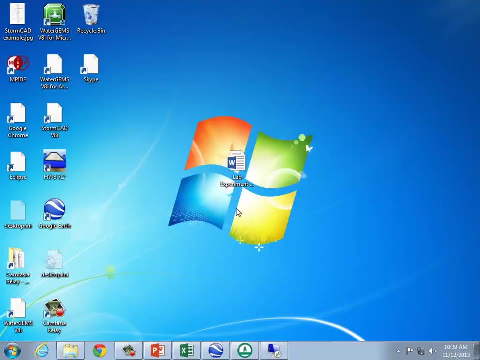 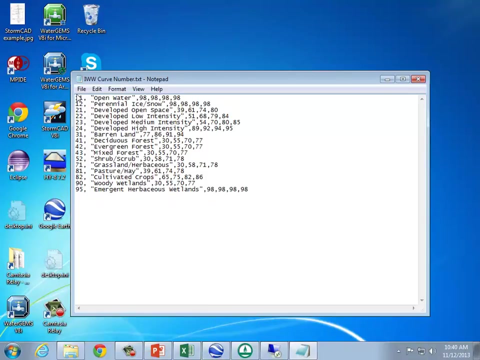 Hmm, Yeah, All right. All right, This is so. in that picture, each of the colors means a different land use type, And so one color will be barren land, Another color will represent developed open space. 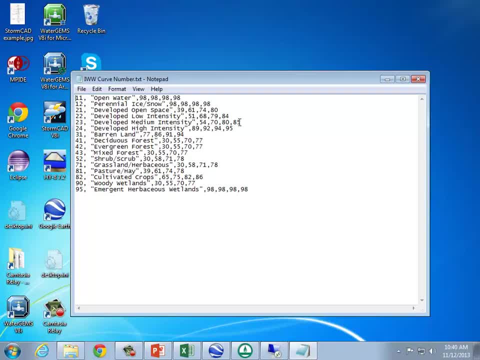 And so on. And then there is a series of numbers after these. What do you suppose these numbers refer to? What's that? They're curve numbers, That's right. Why are there four of them? Those are different soil types. 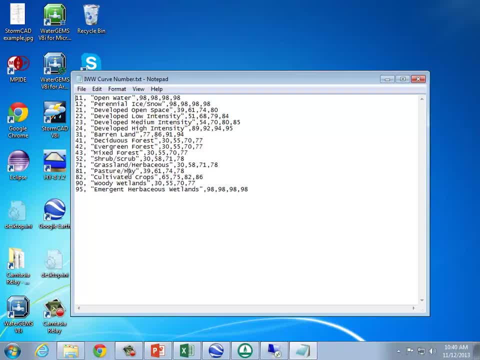 Yeah, So for example, if the land use file says a certain spot is pasture, slash hay, then it has four curve number options. We'll download separately a soil type data that says in that particular area whether it's soil type A, B, C or D. 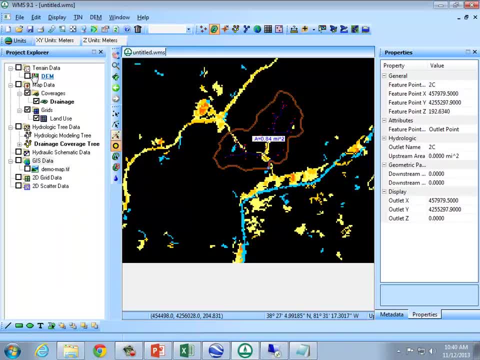 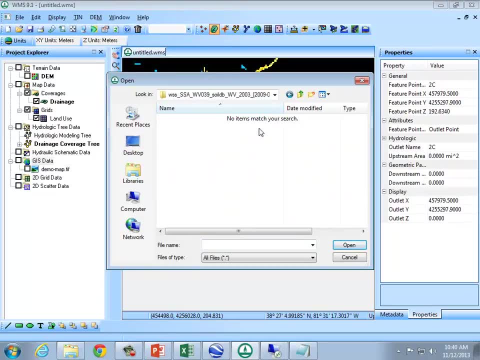 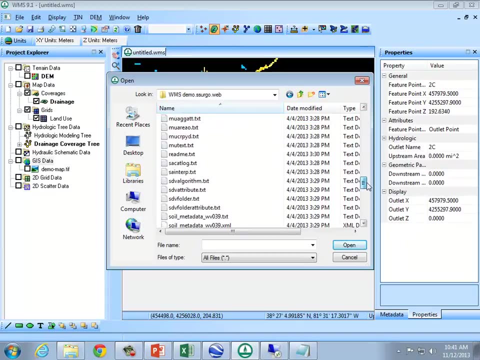 And so now we've got the land use here, Let me see if I can have it open up the soil type that we downloaded. Here's the Sergo soil type- I may be wishful thinking there- Soil A, it's the big one. 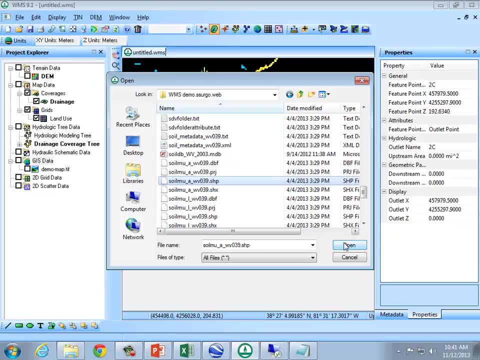 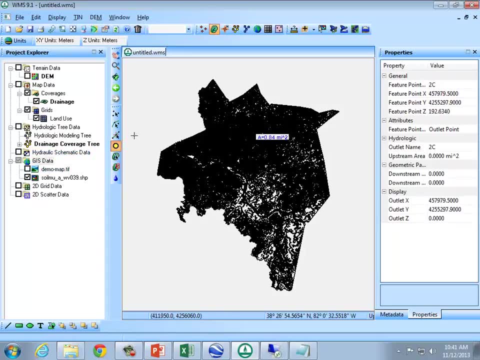 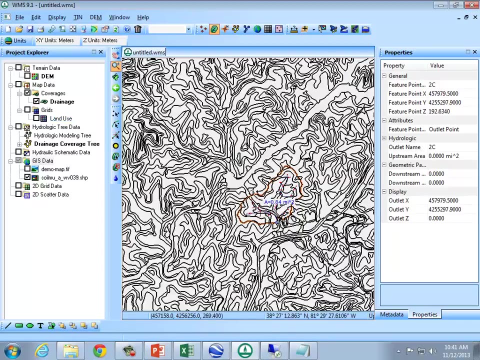 Oh, I think I put it in the wrong spot. Oh there, it is All right, good, Okay, so we turn off the land use. Let's zoom in on our watershed area. So look at it knows the lots of different soil polygons for our 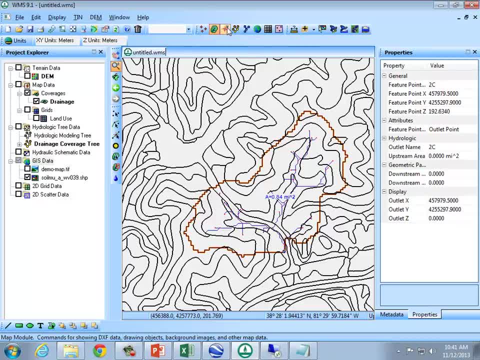 inside of our watershed area And if we go to the GIS module- yeah, If you go to the GIS module, then it'll let. if you click on one of these, one of these shapes, it will tell you what it is. 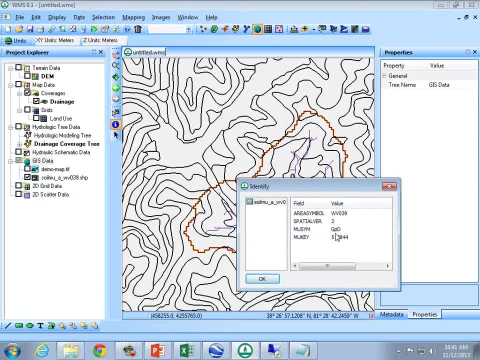 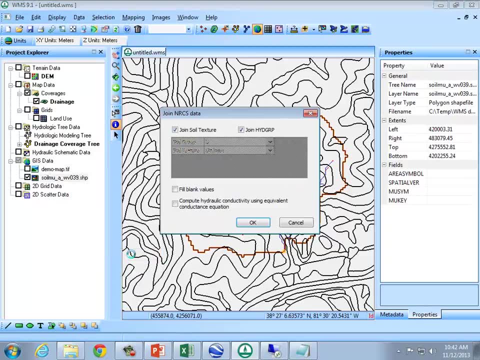 So here I just clicked on a shape and it tells me that it is a GPD, That's like a certain soil type. And if I right click join NRCS data, then it will get the hydrologic group, which is A, B, C, D. 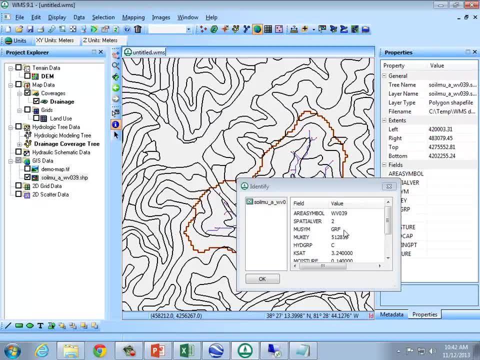 So I need to do that. So when I click on a cell it'll tell me that's hydrologic group C. So this polygon right here is group C, Down there C. This is a lot of C soils in the area. 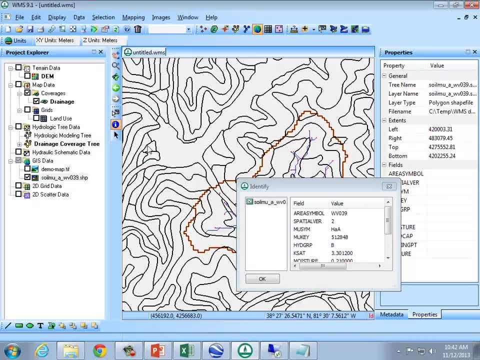 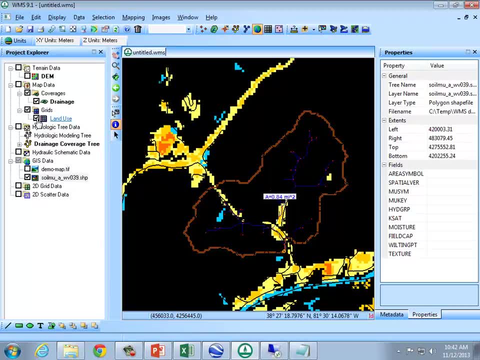 All right, Almost entirely. it looks like There's a B soil right there, that small one. So we have all these soil polygons and on top of it different land use polygons, and it'll automatically calculate the curve number for us. 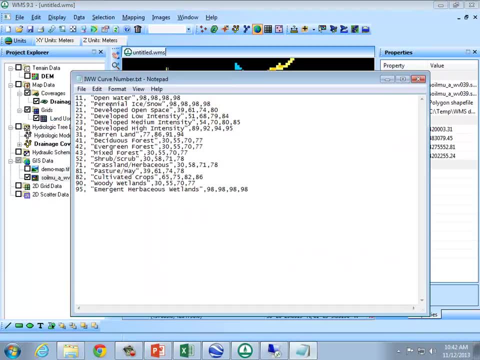 By using this table as the key. So think about it. There's two things going together. There's land use, which is which one of these. you know like which row, any particular spot. The land use file defines which row you're on. 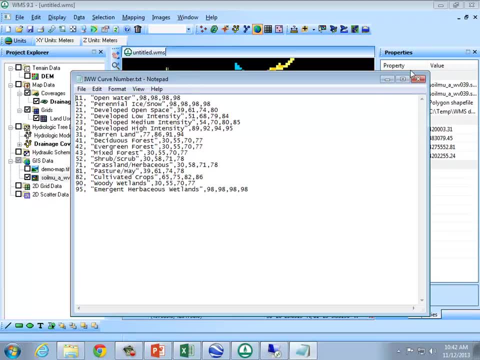 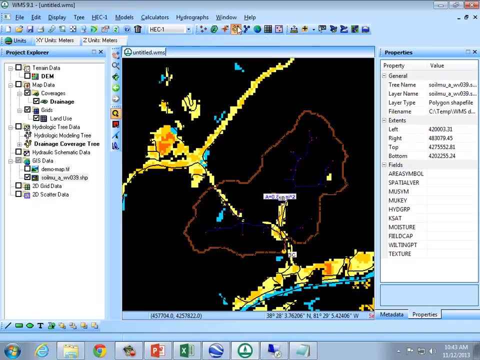 The soil data defines which of the four values that it gets, And then you come up with an aerial weighted average. So let me do that calculation. now I'll go to the hydrologic modeling tool and there's a calculator. Compute GIS attributes. 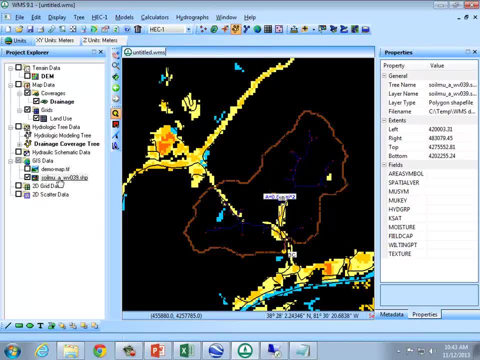 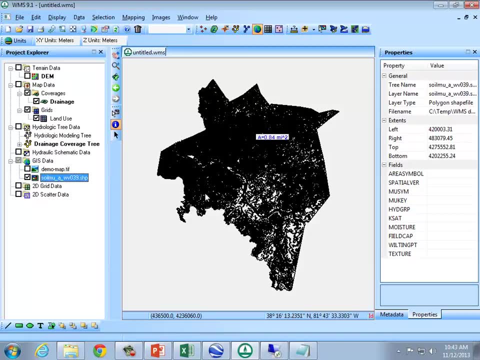 You know, one thing I need to do, though: since this is such a big- you saw how large that is- I probably ought to just select the areas that are inside of our watershed. Otherwise, it's going to take a really long time to compute. 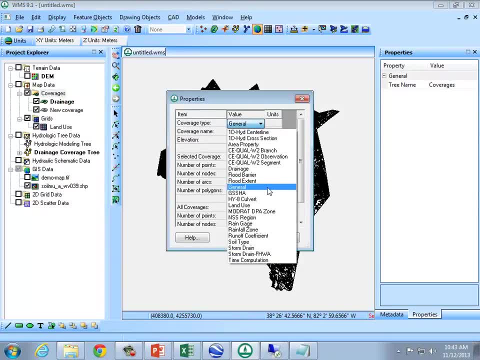 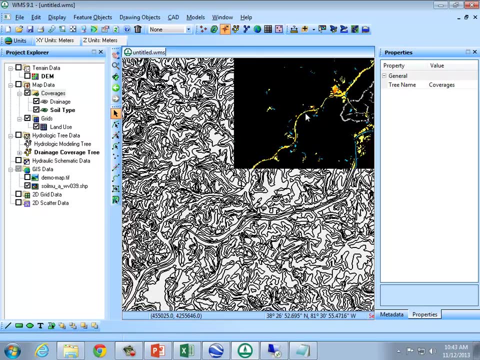 So I'm going to create a new coverage, a soil type coverage. You'll learn how to do all this. There's like a million different steps that I've done today and you don't need to worry about remembering all one million of them. 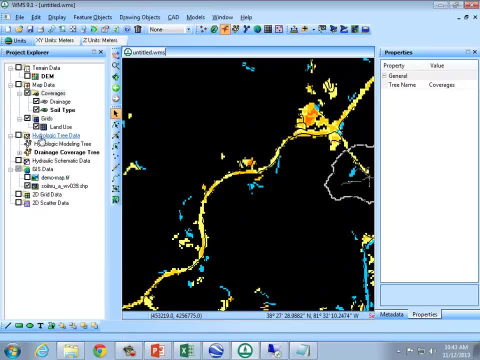 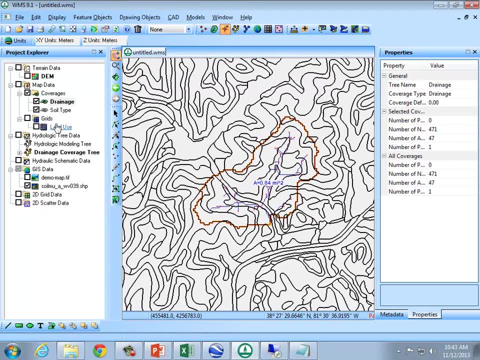 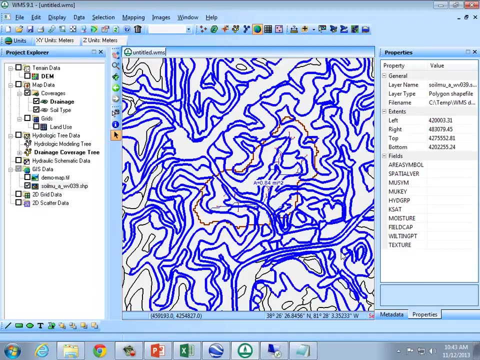 Probably just you know half a million at most that you need to have memorized from today. So let me pan back over to here and I'm going to select only the soil elements that are inside of our Now. a lot fewer of them are selected. 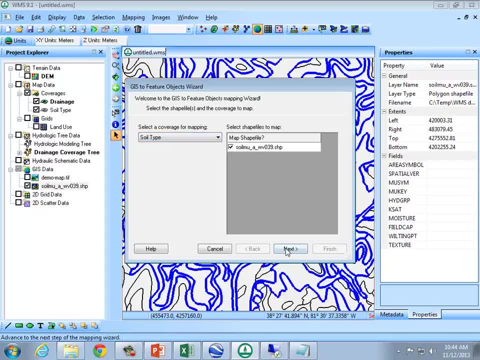 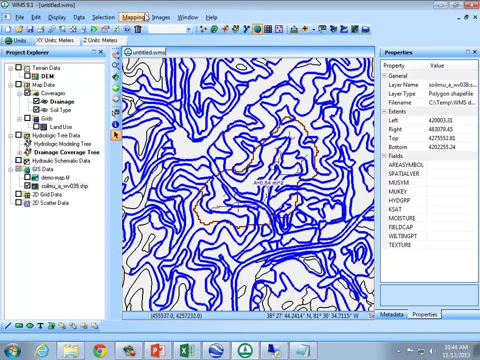 Now I'm going to move that over to this soil coverage And, Okay, there's hydrologic group as part of it All. right now I can do that calculator thing. I'm going to have it automatically calculate the curve number for the watershed. 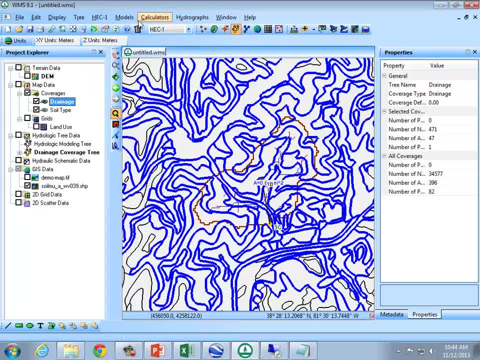 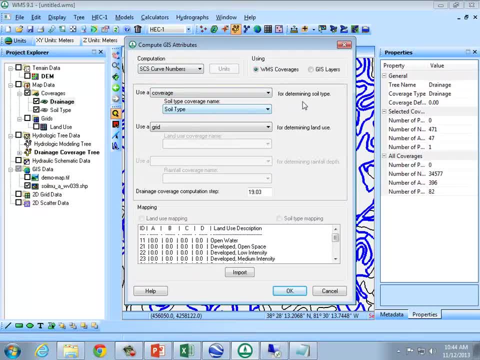 and then we'll be done for today. So I go into the hydrologic modeling module, compute GIS attributes, and so it's going to use the soil type coverage for determining soil type. It's going to use the land use grid for determining land use. 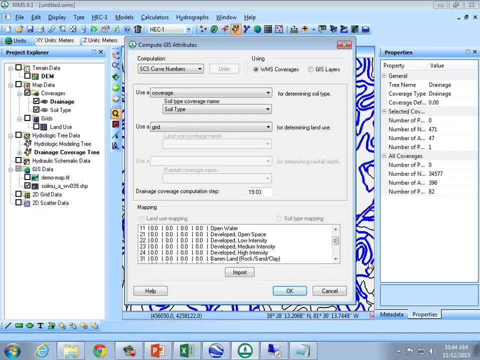 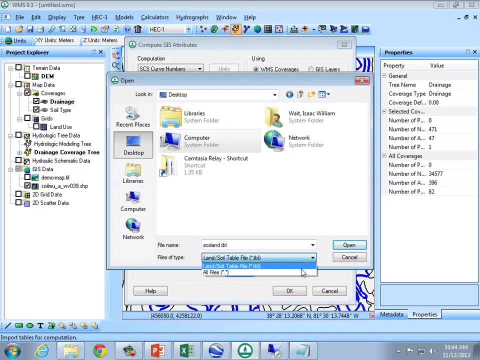 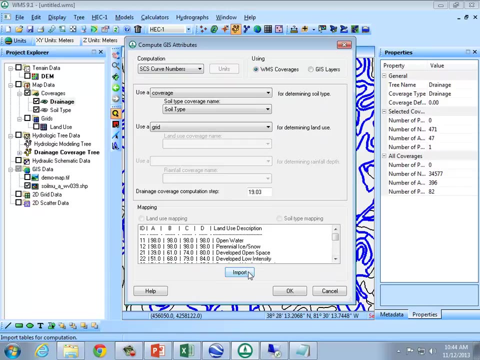 and then it needs to know- like right now it doesn't have any values filled in for that key. So I'm going to import the table that I just pasted onto the desktop. I'm going to use that curve number table And you can see. now it knows all the A, B, C, D land use. 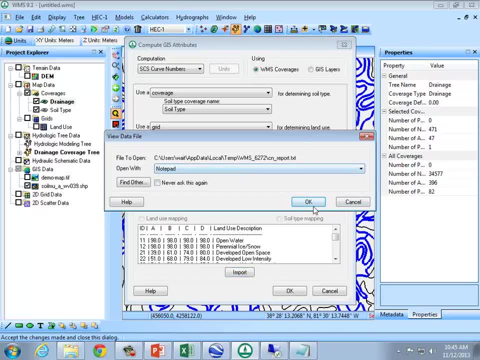 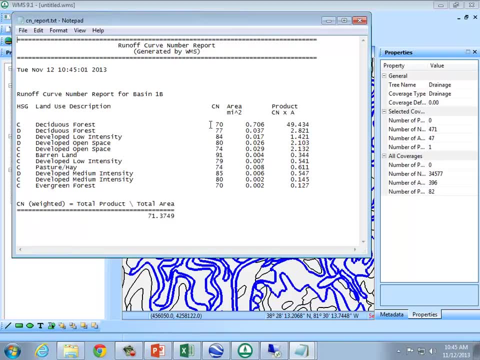 So it does the. It's already finished and it's just offering to bring up the report. So it's calculated the weighted average. It sees that there's some C, some D. you know how much of the area of each part of it. 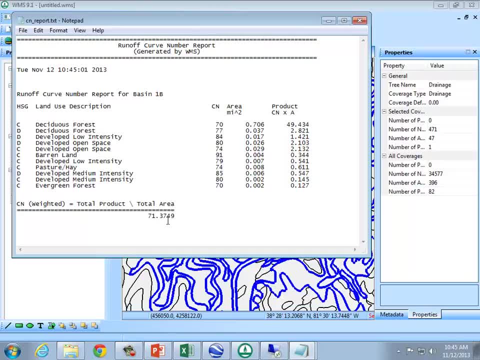 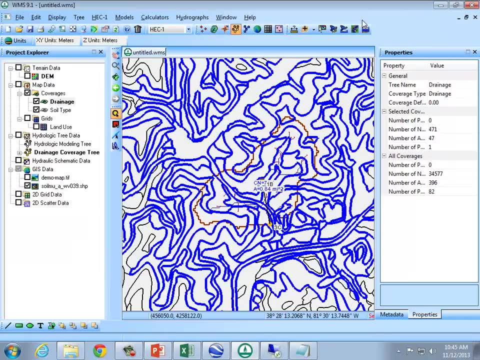 and it comes up with a weighted average of the curve number. So we know the curve number is about 71 for our watershed. So this is sort of the stuff that we're going to work on. Thursday is setting up a watershed model and then Tuesday of next week. 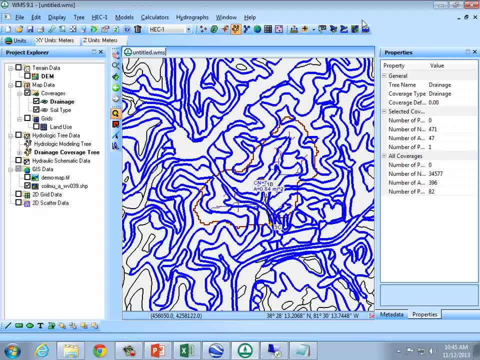 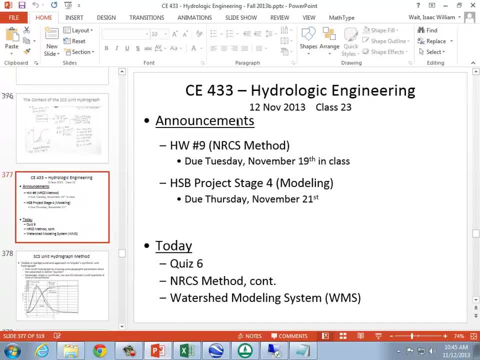 we'll actually be executing the model. So That is it for today. I'll see you on Thursday. Just revisit these announcements. Remember that you've got homework nine with you right now to be working on and, of course, the project as well.